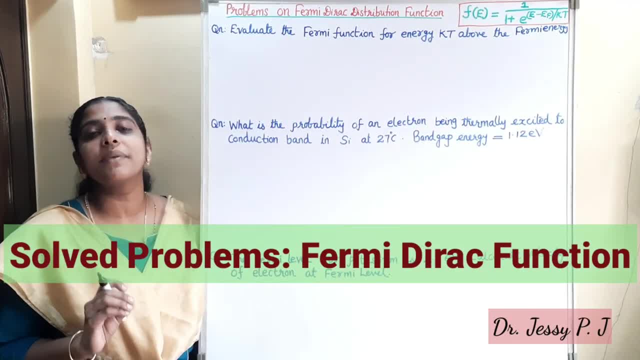 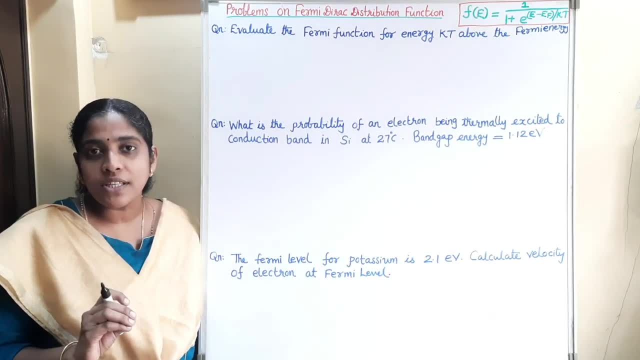 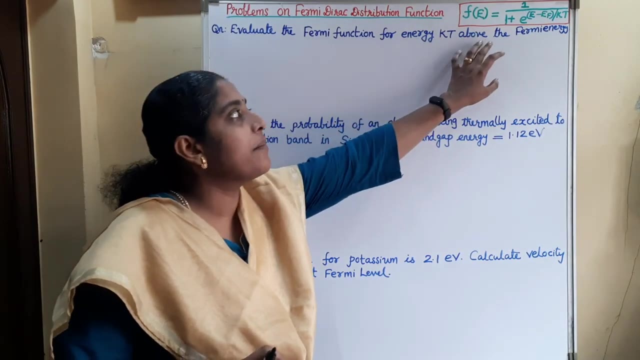 Hi all. today we can see some problems based on Fermi Dirac distribution function. What is Fermi Dirac distribution function in the case? It gives the probability of occupancy of an electron in an energy level It is given by. f of e is equal to 1 by 1 plus e raised. 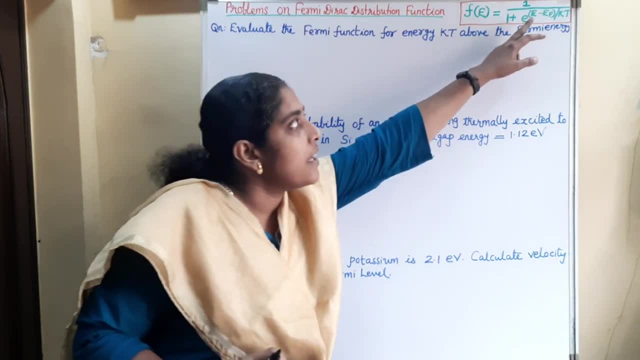 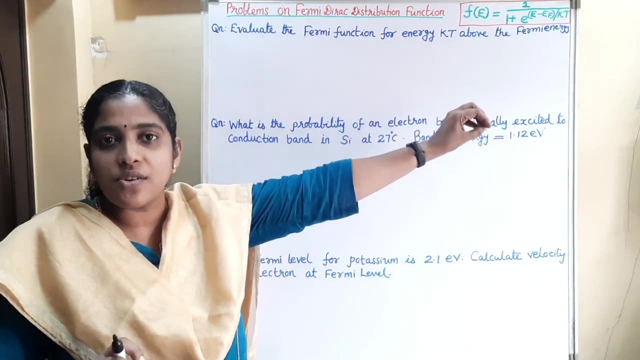 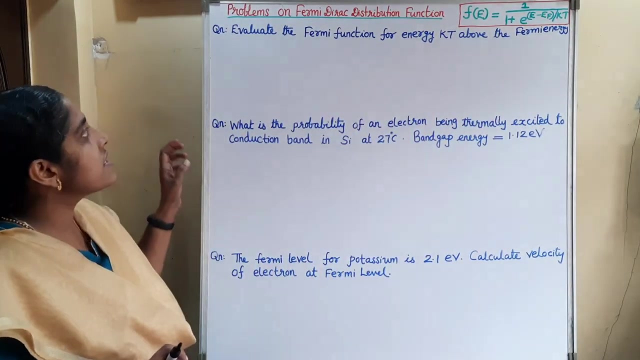 to e minus ef by kt, where e is the energy level in which we are finding the probability of occupancy, Ef is a reference energy level that is known as Fermi energy level, k is the Boltzmann constant and t is the temperature in Kelvin. So see the first question. Evaluate. 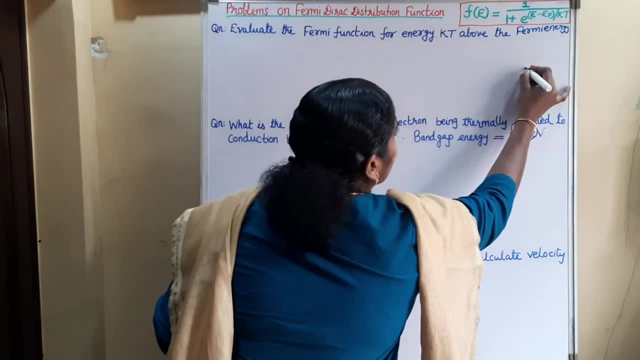 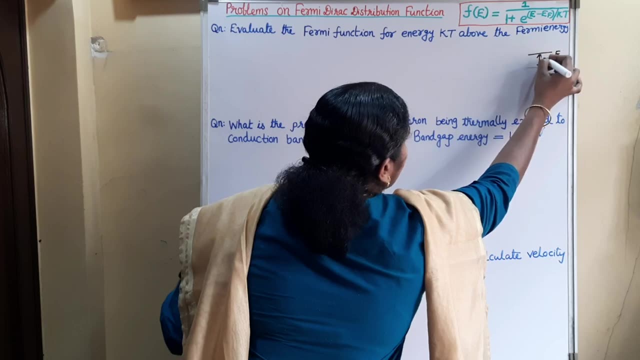 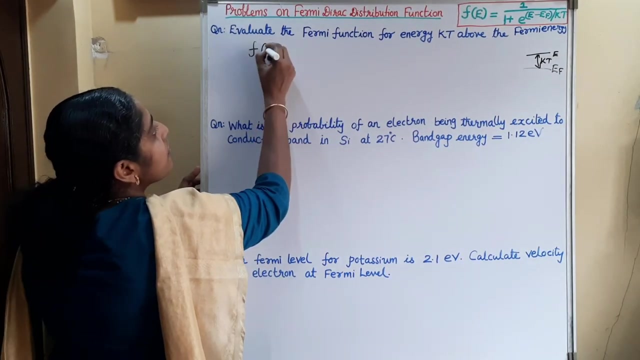 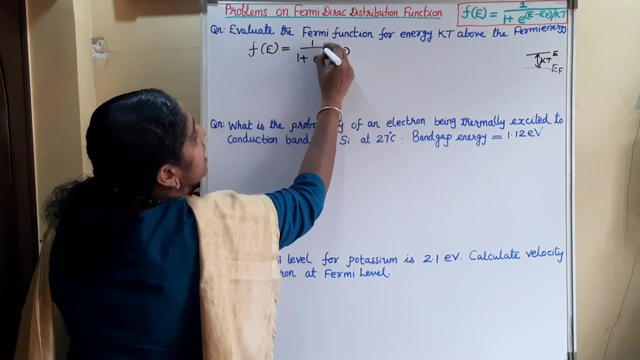 the Fermi function for energy, kt above the Fermi energy. So we have an energy level e. That energy level is kt above the Fermi energy. So here we can find out the Fermi function from that general formula That is, f of e is equal to 1 by 1 plus e, raised to e minus ef by kt. So what is e minus ef? 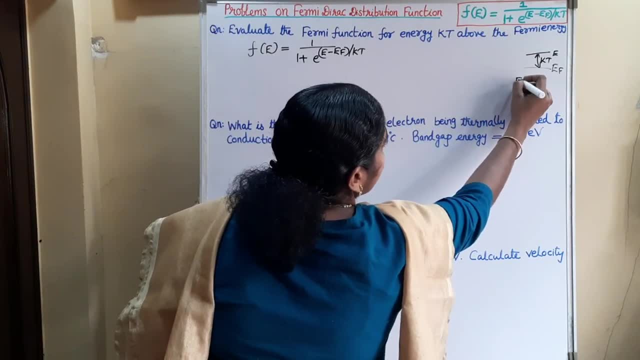 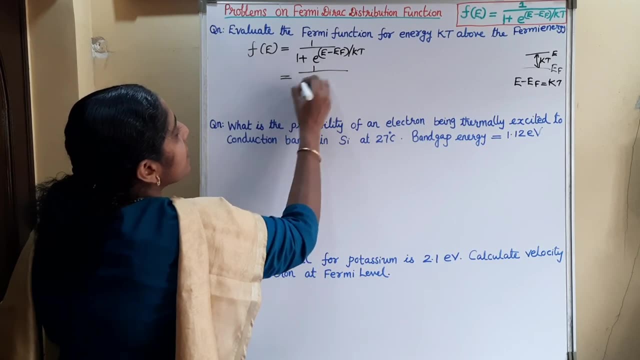 here Where the energy level is kt above ef. So e minus ef is equal to kt. The difference is kt, So we can substitute here 1 by 1. plus e raised to e minus, ef is kt by kt. That is. 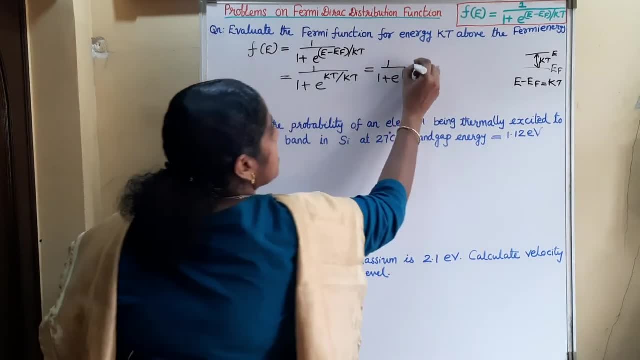 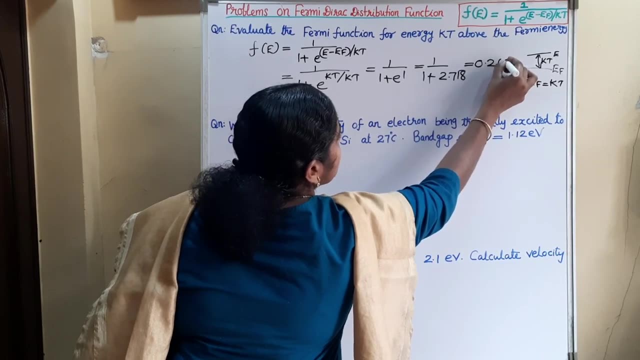 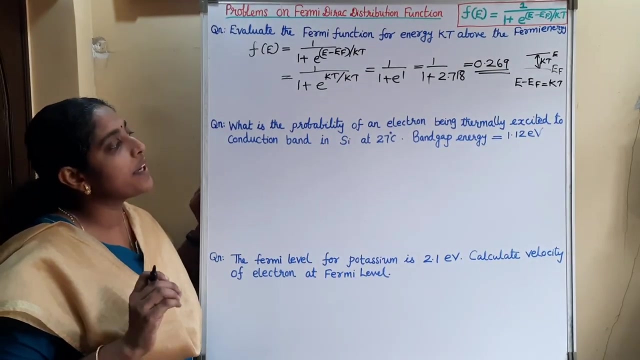 1 by 1 plus e, raised to 1.. That is 1.. So 1 by 1 plus 2.718.. On calculating we will get 0.269.. So the Fermi function is 0.269.. Now see the second question: What is the probability of an electron being thermally? 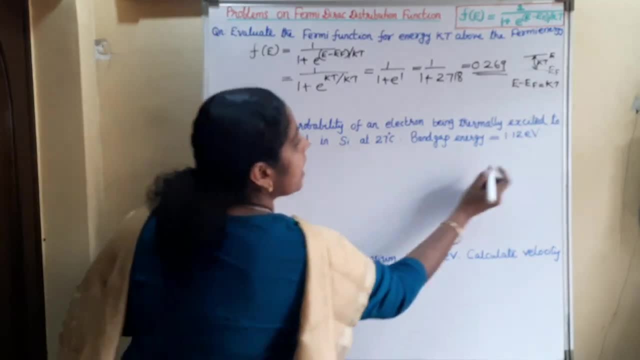 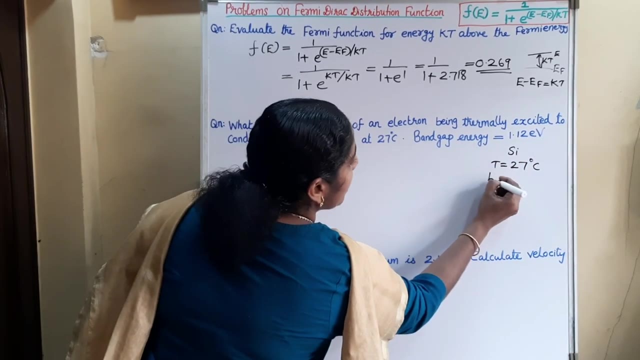 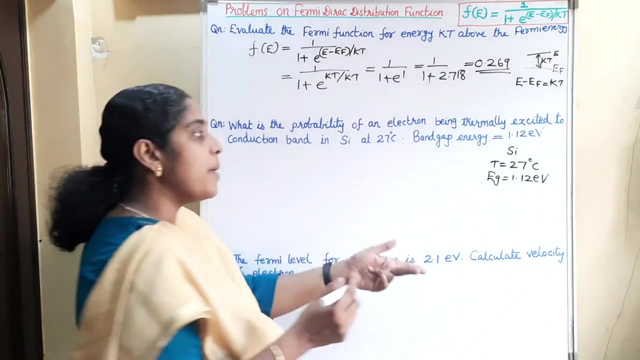 excited to conduction band in silicon at 27 degree Celsius. So temperature is equal to 27 degree Celsius. It is given that band cap energy is 1.12 electron volt. So what we have to find out? We have to find out the probability That means f of 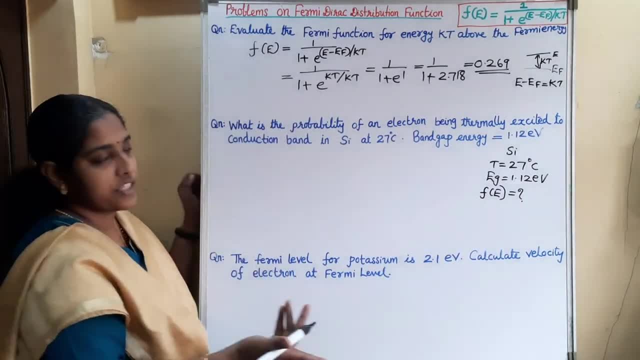 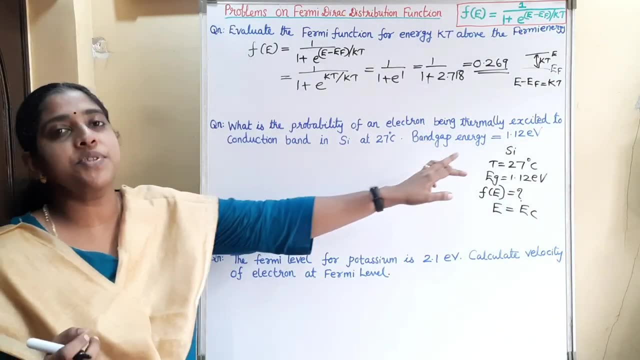 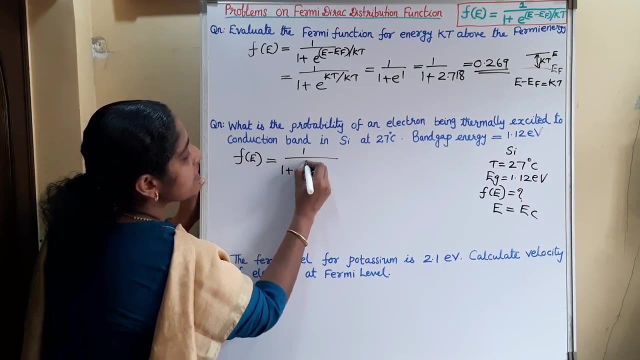 e that is being thermally excited to conduction band. So the energy level e here is the conduction band, energy, So we can substitute this data in the general formula, That is, f of e is equal to 1 by 1 plus e, raised to e minus ef by kt. So here the energy level is conduction. 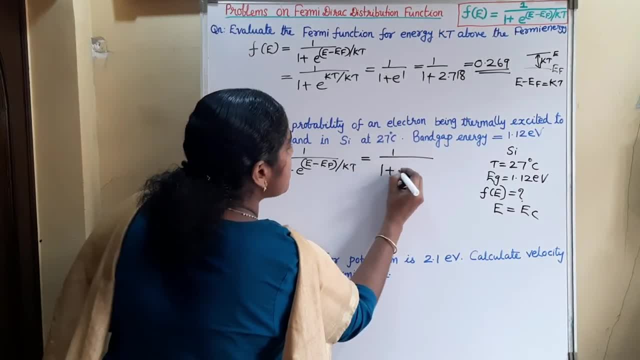 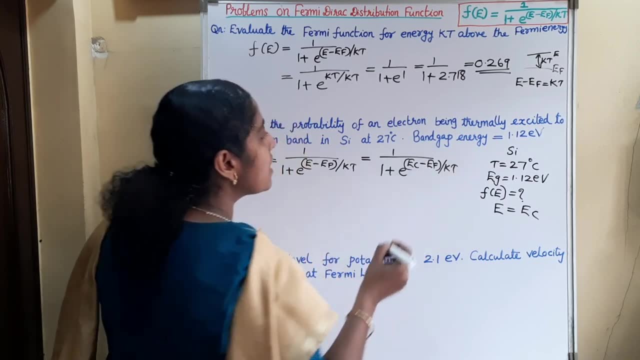 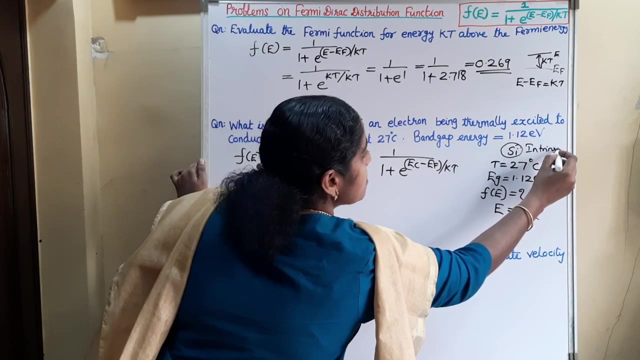 band energy. so that is 1 by 1 plus e, raised to conduction band energy, minus ef by kt. now the given material is silicon. silicon is an intrinsic semiconductor. so in the case of intrinsic semiconductor, what is the difference between conduction band energy and fermi energy? 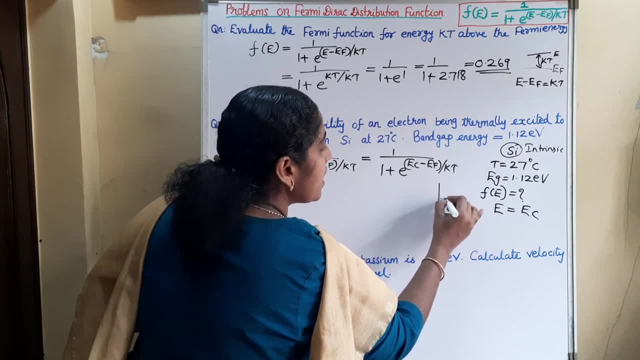 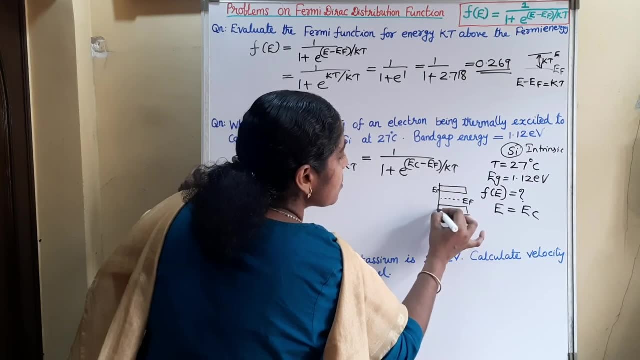 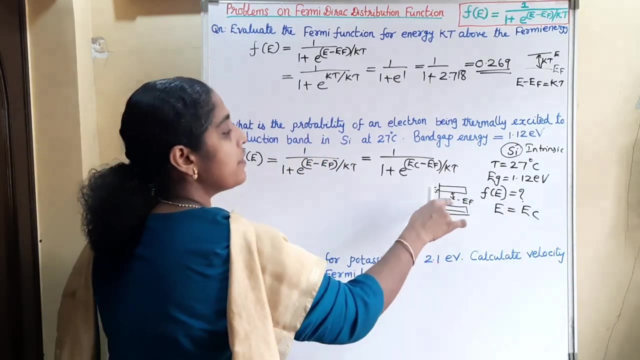 in intrinsic semiconductor the fermi level lies in the middle of conduction band and the valence band. so this gap is that is, the difference between conduction band and fermi level. and also the difference between valence band and fermi level is the half of the energy gap. so in this 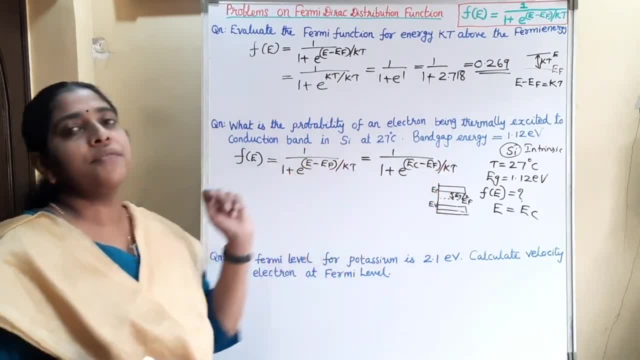 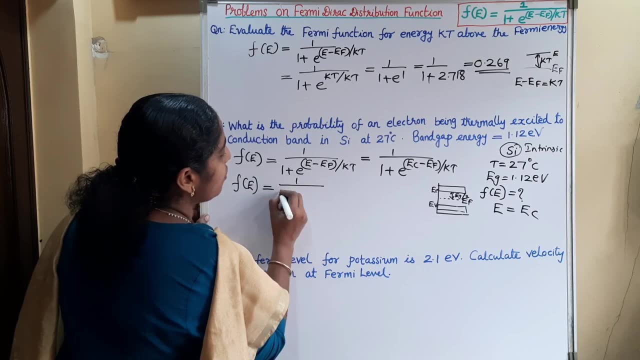 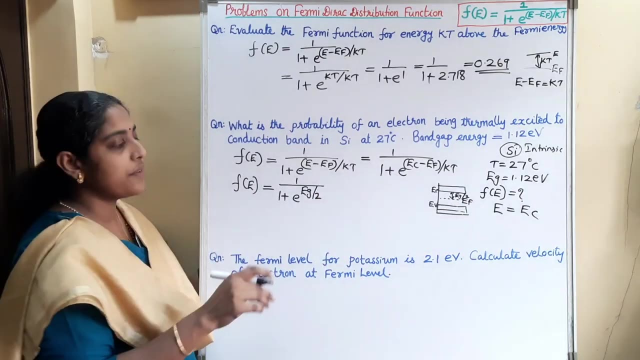 case we can write the difference between conduction band and fermi level as the half of the energy gap, that is fermi function. fov is equal to 1 plus e. raised to eg by 2, that is ec minus ef, is the half of the energy gap, and already kt is there. okay, now we can. 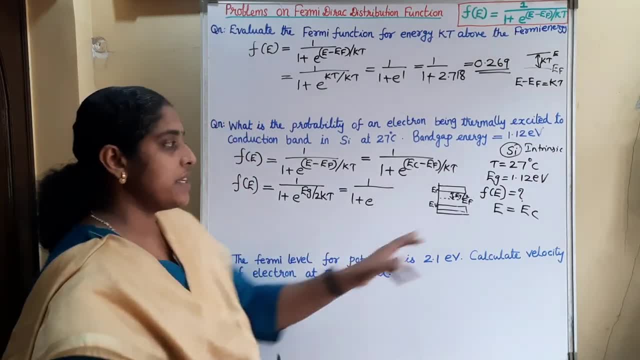 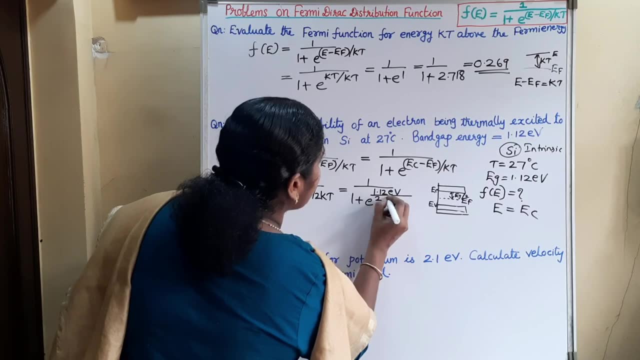 substitute 1 by 1 plus e raised to eg, that is, energy band gap is given 1.12 electron volt divided by 2 into k. k is the Boltzmann constant. now here, remember that k is the Boltzmann constant. so we can substitute 1 by 1 plus e raised to. 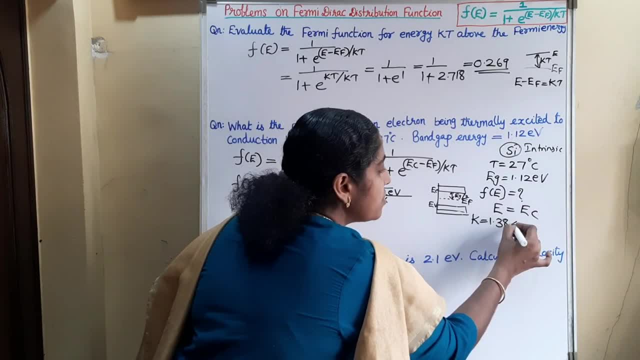 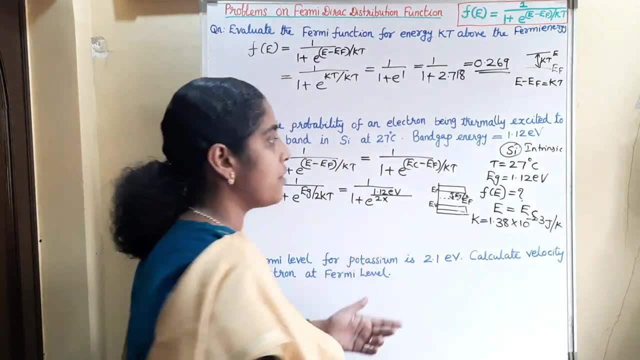 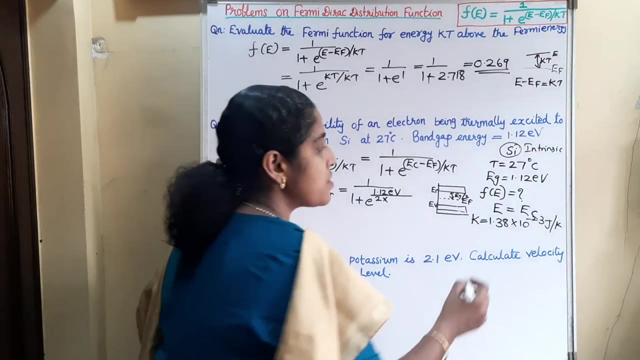 eg by 2.. now remember, the Boltzmann constant value is 1.38 into 10, raised to minus 23 joules per kelvin. now for simplicity, we can use the Boltzmann constant in electron volt to find this joule to electron volt. divide this by 1.6 into 10, raised to minus 19. so on converting. 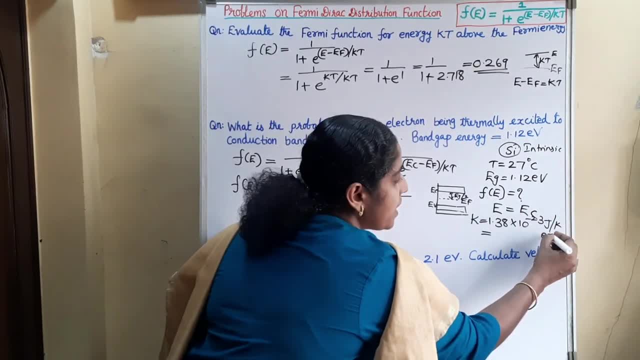 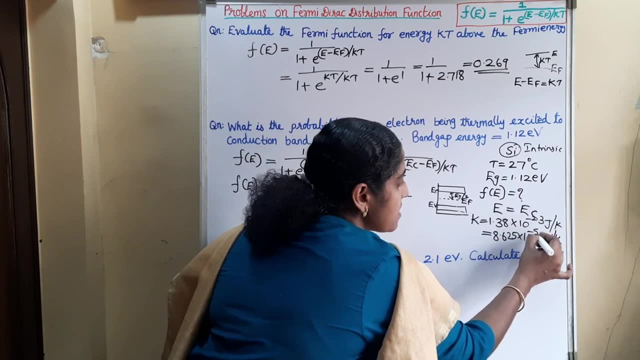 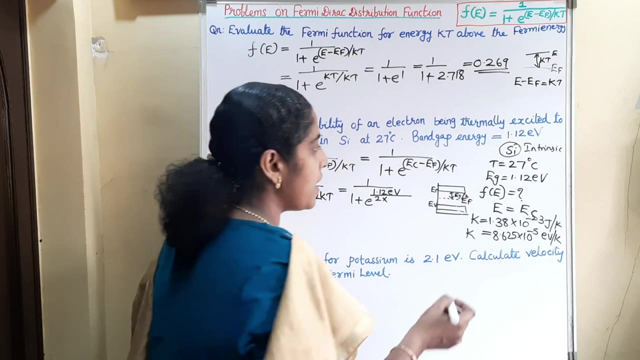 this joule per kelvin to electron volt per kelvin, we will get 8.625 into 10, raised to raise to minus 5. that is Boltzmann constant into unit of electron volt per Kelvin is 8.625 into 10 raise to minus 5.. Now the temperature. temperature is 27 degree Celsius. So we have to. 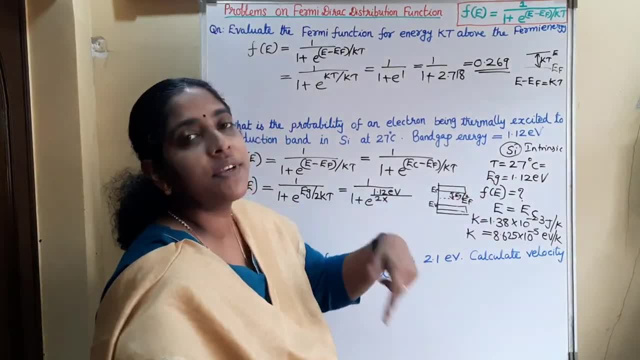 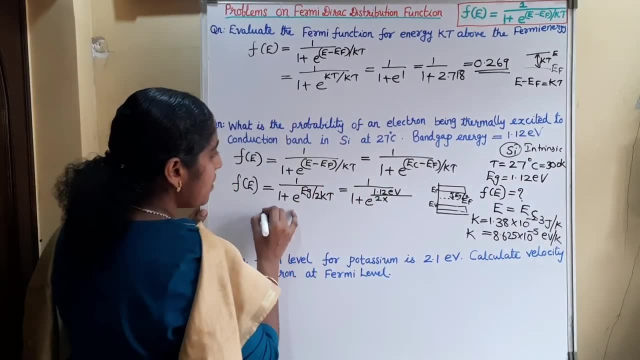 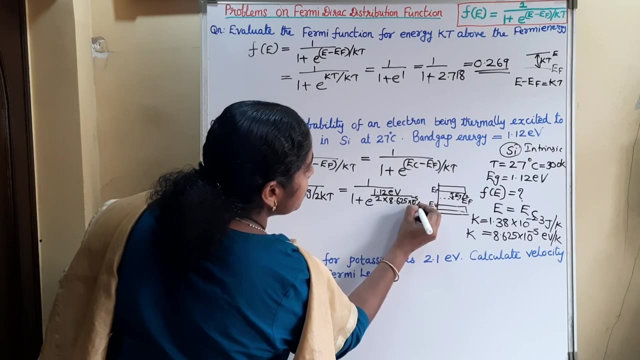 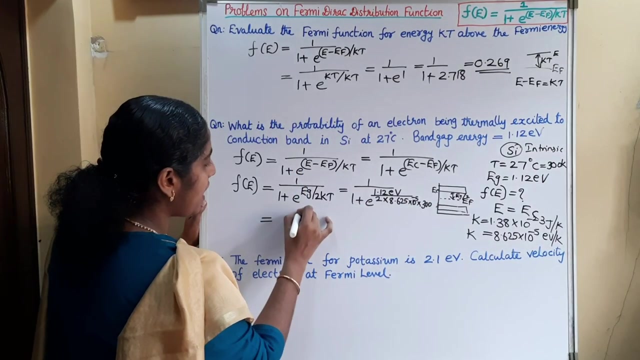 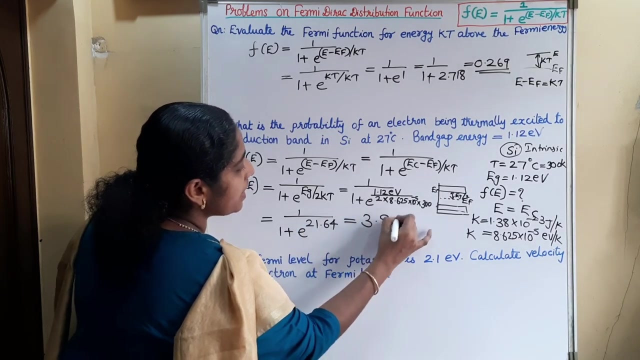 write this in Kelvin, So Celsius we can convert into Kelvin by adding 273, that is 300 Kelvin. So substituting here it is Boltzmann constant is 8.625 into 10. raise to minus 5 into this temperature, that is 300.. On solving this we will get 1 by 1 plus e raise to 21.64, that is 3.998. 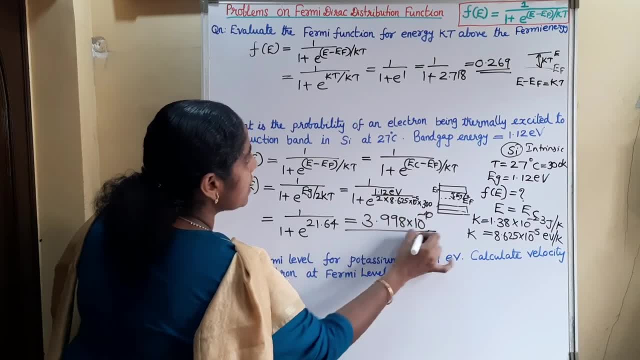 into 10, raise to minus 10.. So here the probability of an electron volt per Kelvin is 8.625 into 10 raise to minus 5.. So substituting here it is Boltzmann constant into unit of electron volt per Kelvin is 8.625 into 10, raise to minus 5.. So here the 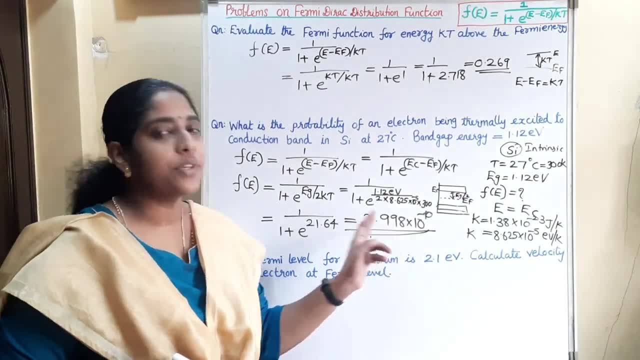 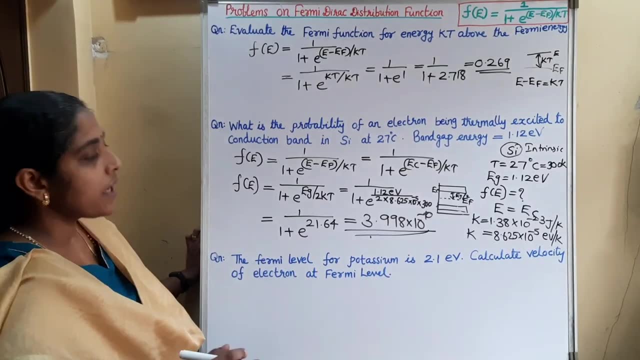 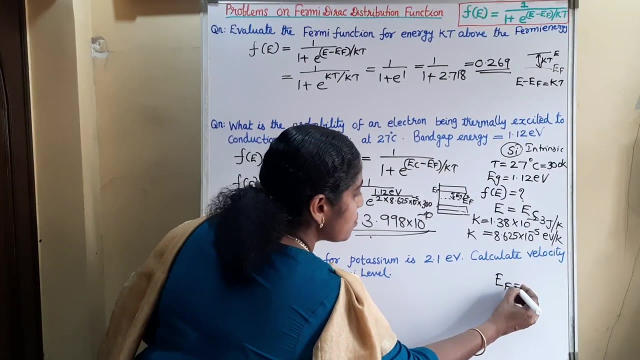 thermal excited to conduction band is 3.998 into 10, raise to minus 10.. See this question. the Fermi level for potassium is 2.1 electron volt. Calculate velocity of electron at Fermi level. So here the Fermi level is given as 2.1 electron volt. Calculate the velocity of electron at Fermi level. 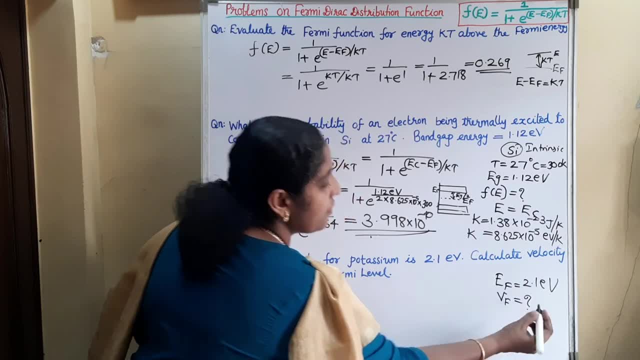 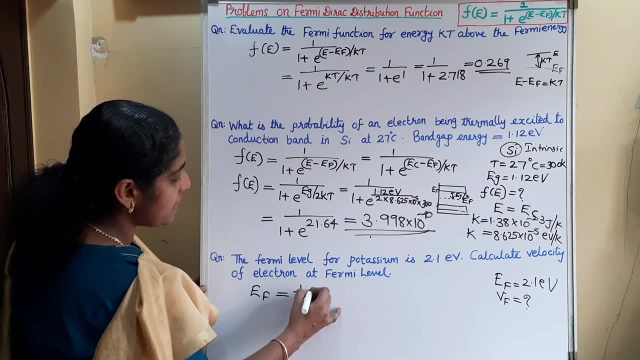 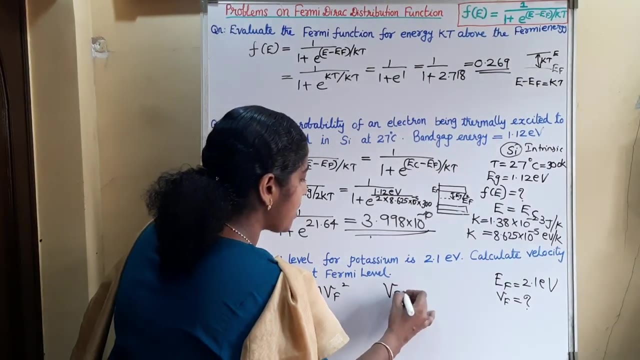 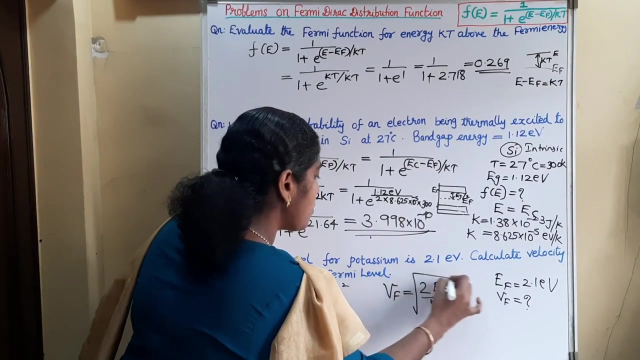 that is, we have to find out the VF velocity of electron at Fermi level. So here we can find the velocity by the general equation of kinetic energy, that is, EF is equal to half m VF square. So VF is equal to velocity of electron at Fermi level is equal to 2 EF by m. and take the. 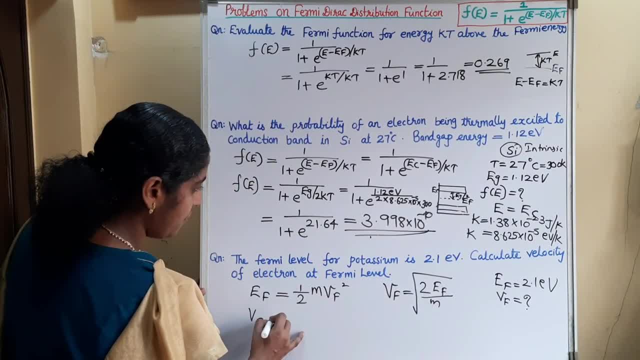 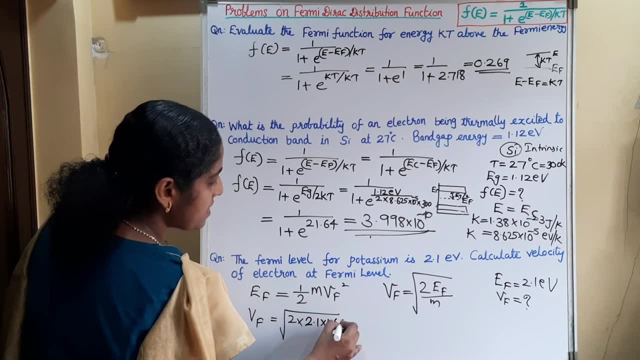 square root, that is VF, is equal to root of 2 into EF, is 2.1 electron volt, that is 2.1 into 1.6 into 10, raise to minus 5 into 10, raise to minus 5.. So here we can find the velocity by the general equation. 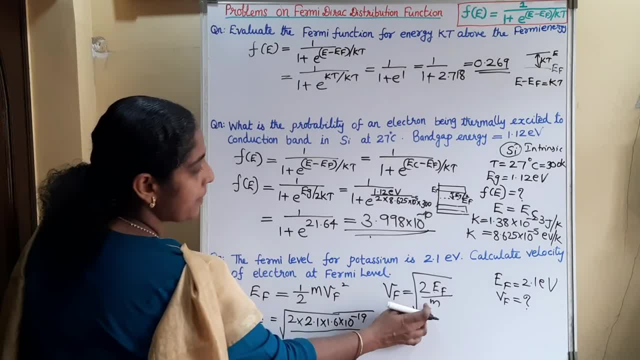 of electron at Fermi level. So here the Fermi level is given as 2.1 electron volt. Calculate the velocity by: the general equation of electron at Fermi level is equal to half m. VF by m into 10. raise to minus 19 joule divided by m. m is mass of electron, that is 9.1 into 10. raise to minus 31.. 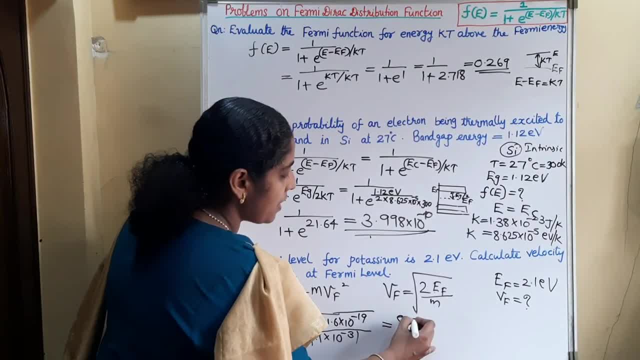 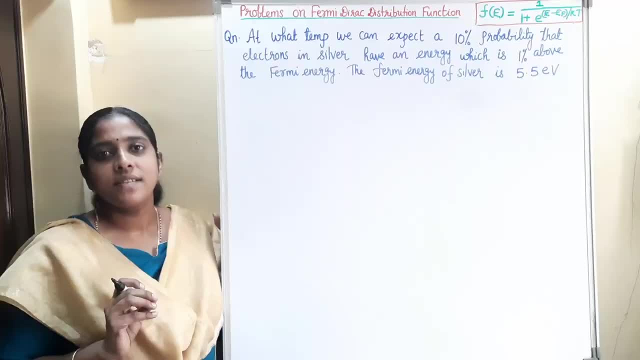 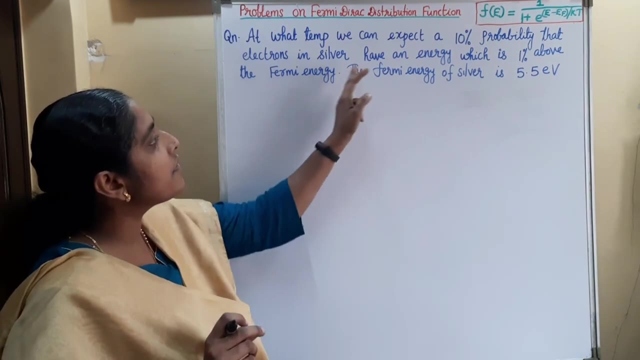 On calculating this we will get 8.59 into 10 raise to 5 meter per second. See the next question: at what temperature we can expect a 10 percentage probability that electrons in silver have an energy which is 10 percent. So here we can calculate the velocity. 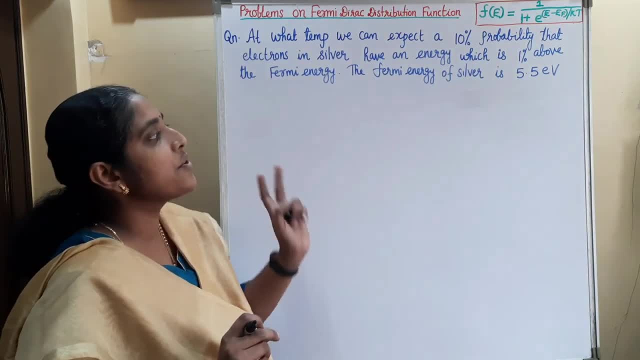 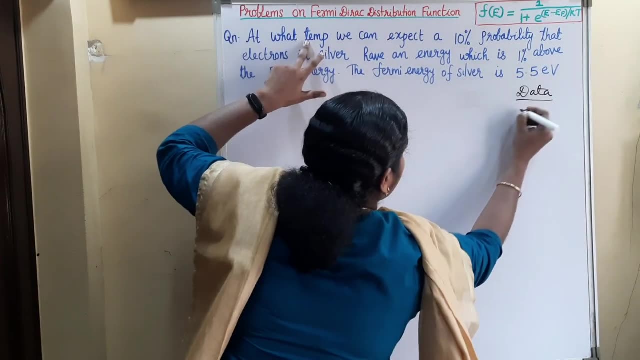 by the generators of the electron at F of compar location. So for the instant energy, the velocity in the�minous is 1이고 is equal toide20 units. So we have to find out the perfect, our Hercher, at what temperature we can expect it and fault in this probability. that is the 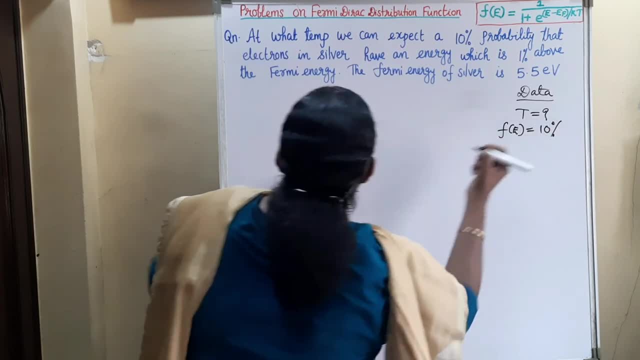 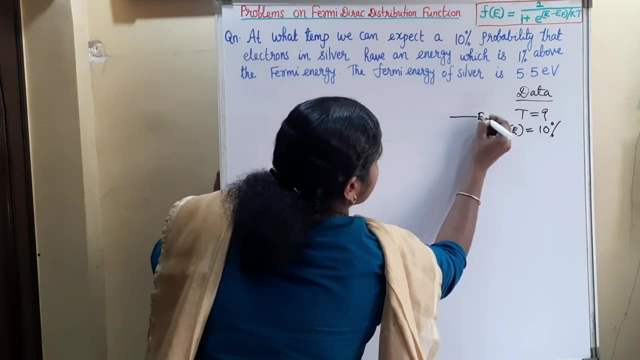 function. a full fee is equal to 10. pas into that illitこと in silver. have an energy which is one person, yet a boat. for me energy code is EF, then the corresponding energy he is căp at F is equal to E Omar, where the name for the EF corresponding energy case. 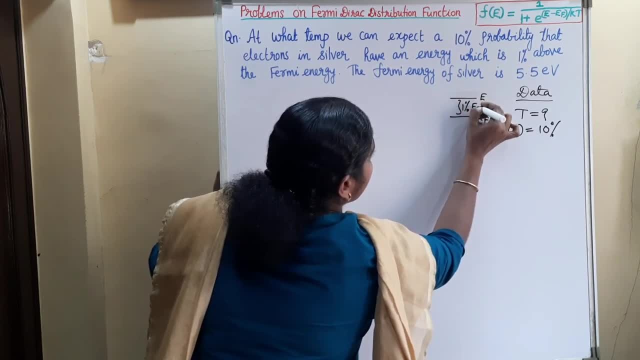 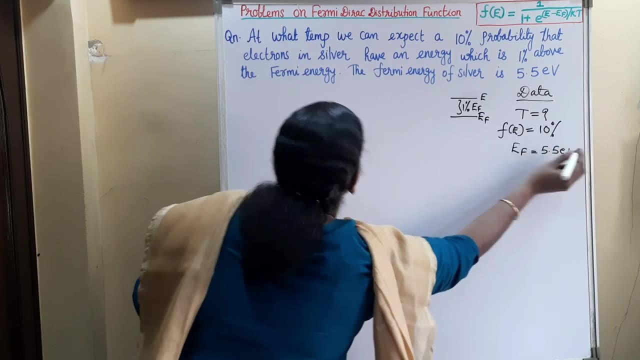 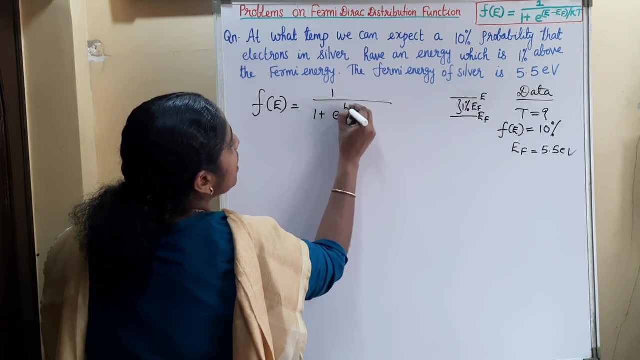 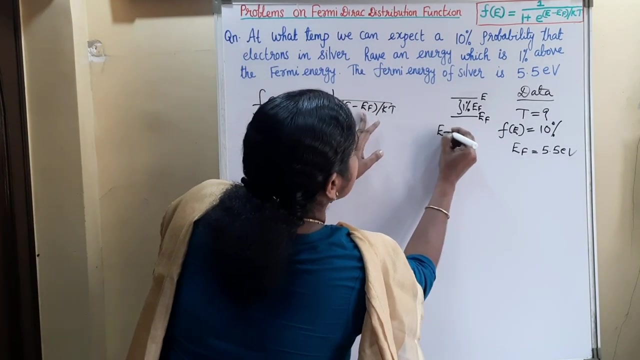 E is căpcak one percentage above the Fermi level. Here the Fermi energy of silver is given as 5.5 electron volt. So we can write the general formula for the Fermi function that is: f of e is equal to 1 by 1 plus e. raised to e minus ef, divided by kt, What is e minus ef? e minus ef is equal to: 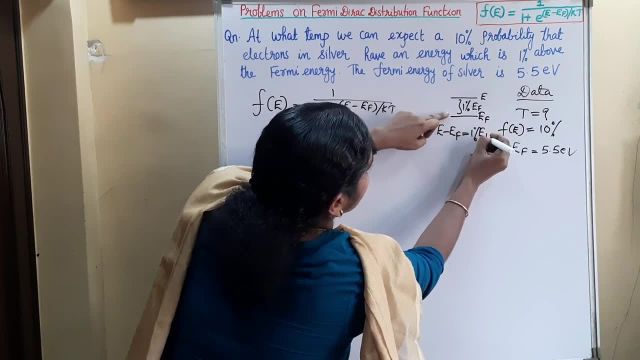 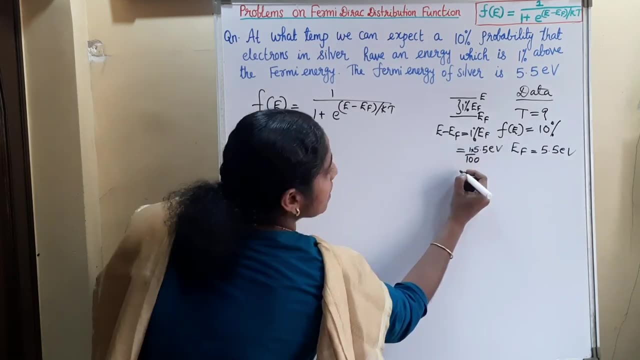 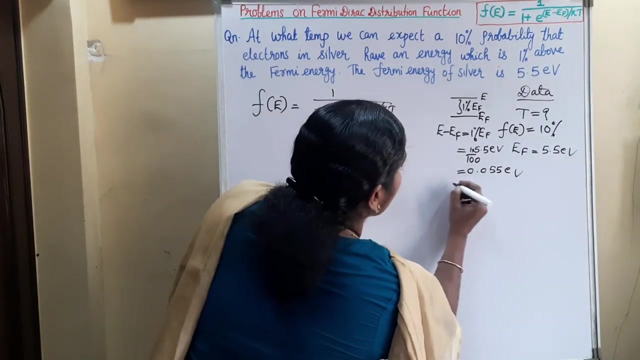 1 percentage of ef. That is 1 percentage of ef is 5.5 electron volt. That is 0.055 electron volt. Next, k, k is the Boltzmann constant. that is equal to 1.38 into 10 raised to minus 23. 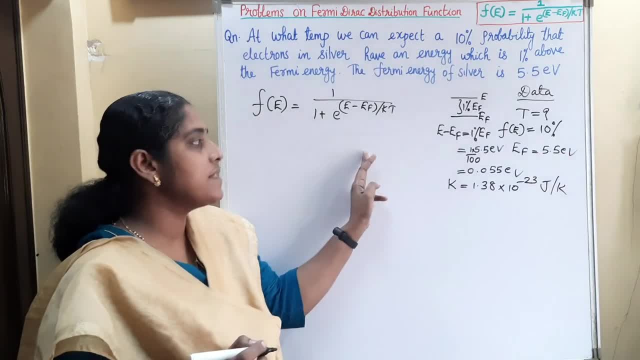 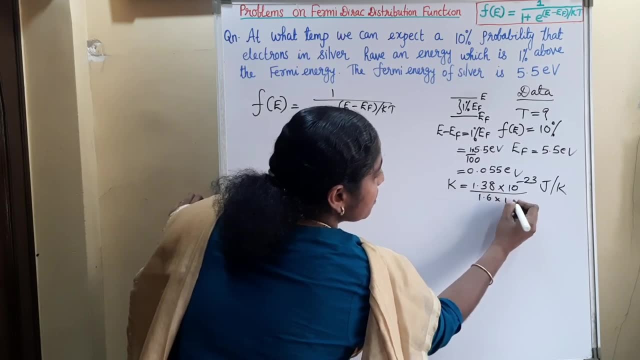 joule per Kelvin. But while doing this type of numericals it is easy if we are writing the Boltzmann constant in electron volt, For that we have to divide it by 1.6 into 10, raised to minus 19. Then we can write it as: 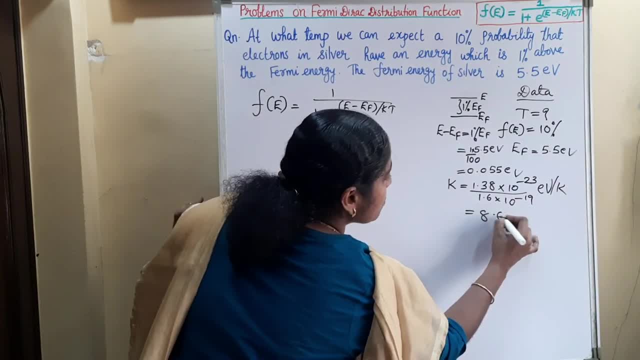 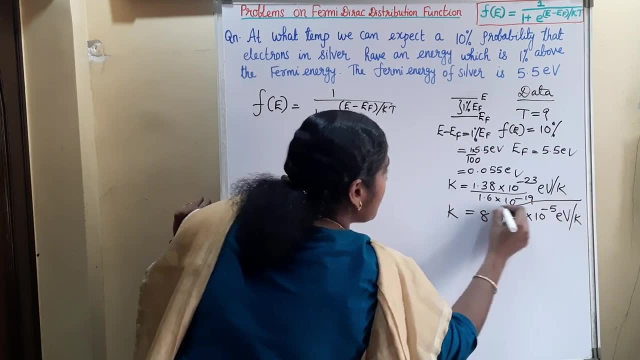 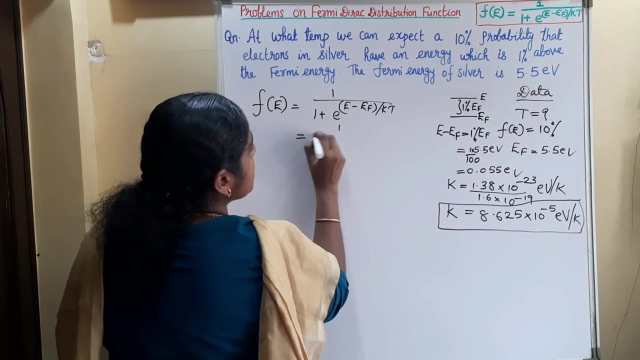 electron volt per Kelvin. So it is 8.625 into 10 raised to minus 5 electron volt per Kelvin Better. you remember this Boltzmann constant in electron volt per Kelvin. that is 8.625 into 10 raised to minus 5 electron volt per Kelvin. So we can substitute here 1 by 1 plus e raised to. 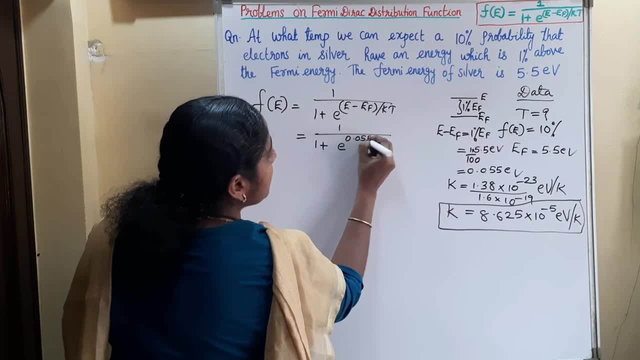 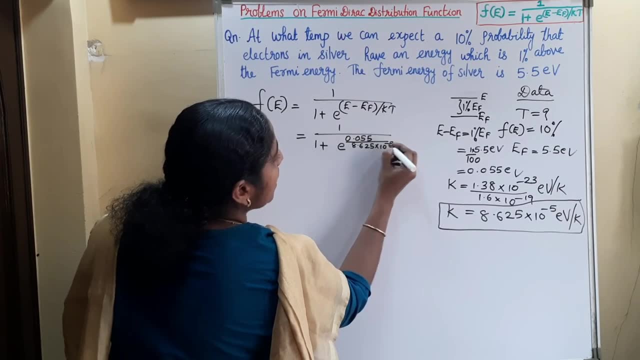 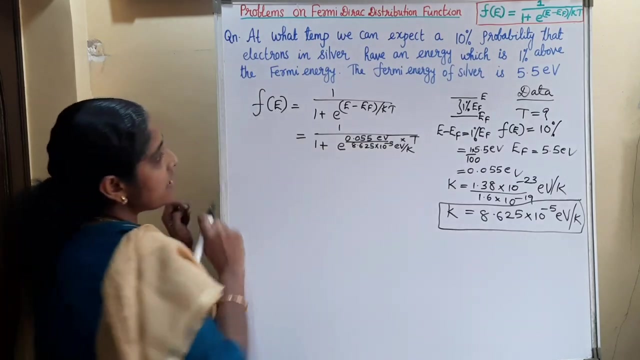 e minus ef is 0.055.. electron volt divided by k is 8.625 into 10, raised to minus 5 electron volt per Kelvin, Here it is electron volt into temperature. So what is f of e here? f of e is 10 percentage. 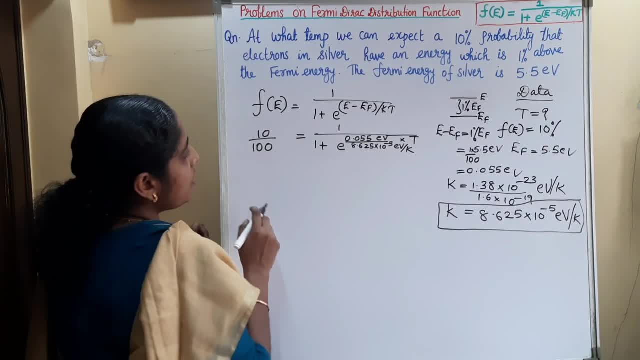 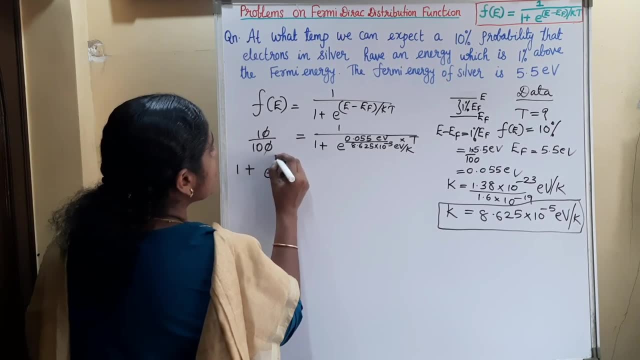 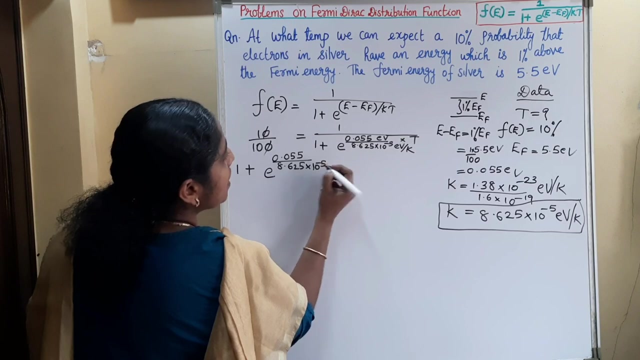 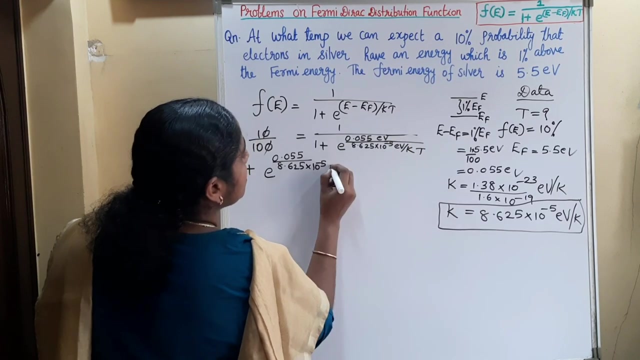 That is 10 by 100.. So this become 1 by 10 and on cross multiplying we will get 1 plus e raised to minus 2, divided by 8.625 into 10, raised to minus 5, into t- Here it is t Okay. Into t is equal to 10.. 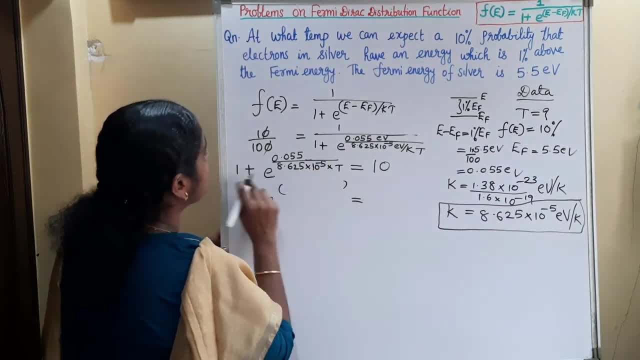 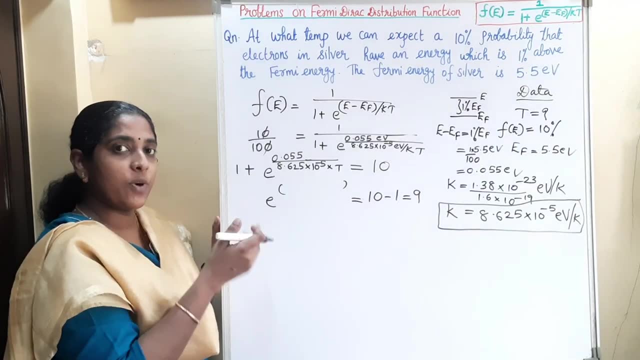 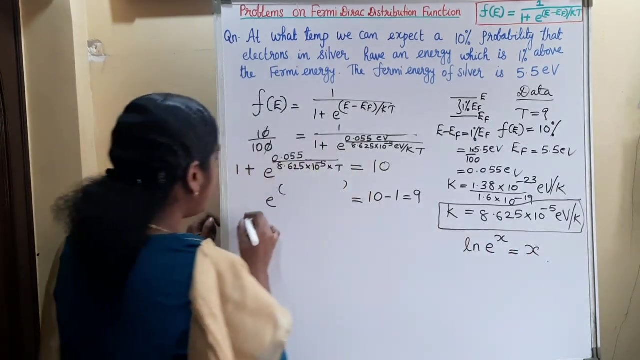 That is, e raised to this term is equal to 1. we can take to RHS, So that is 10 minus 1, that is equal to 9.. We can remove this exponential function by taking the logarithm, because log e raised to x is equal to x. So we can take the logarithm on both sides. So this is log e raised. 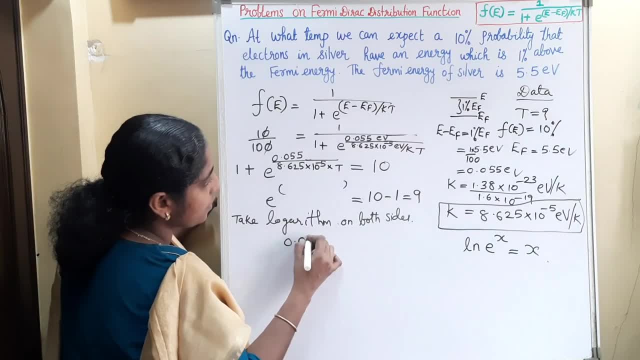 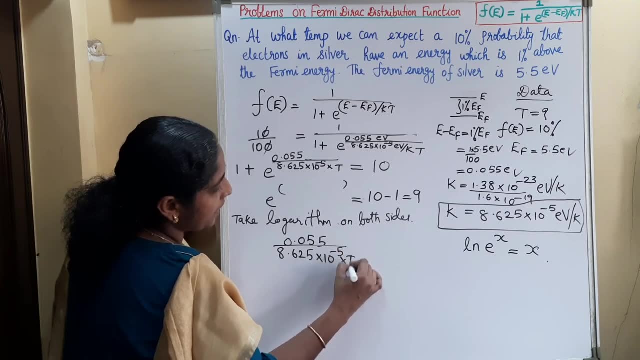 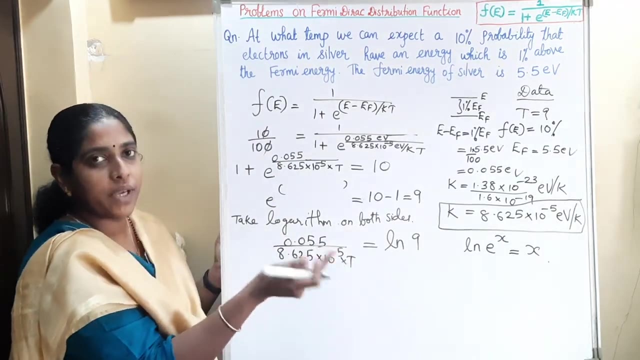 to this term. that is, 0.055 divided by 8.625 into 10, raised to minus 5 into temperature, is equal to log 9.. Take the natural logarithm. If you are taking the logarithm to the base 10, you have to. 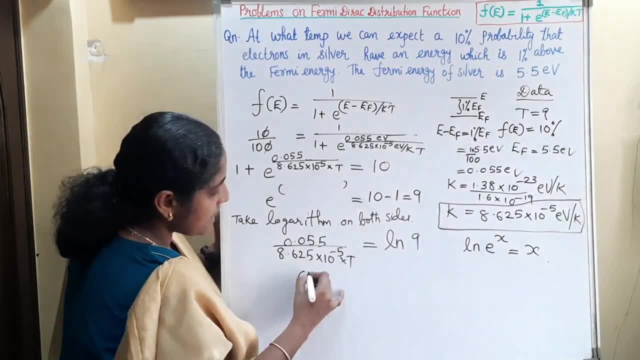 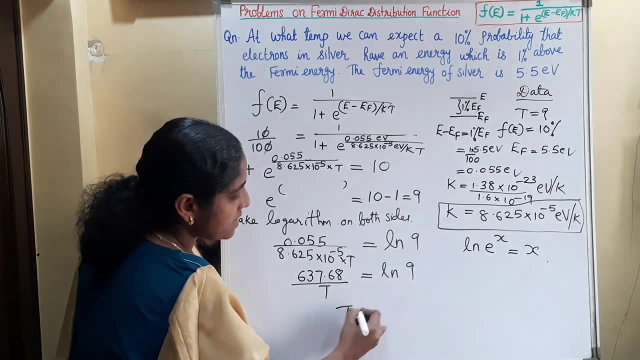 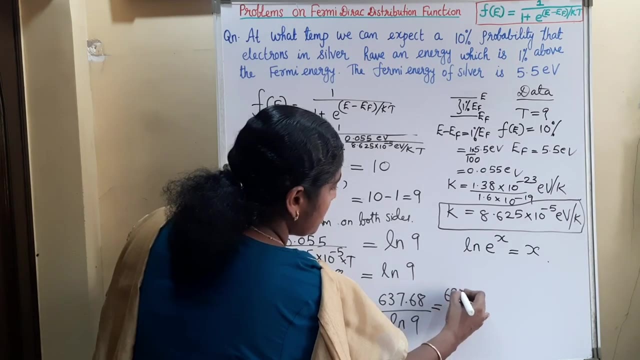 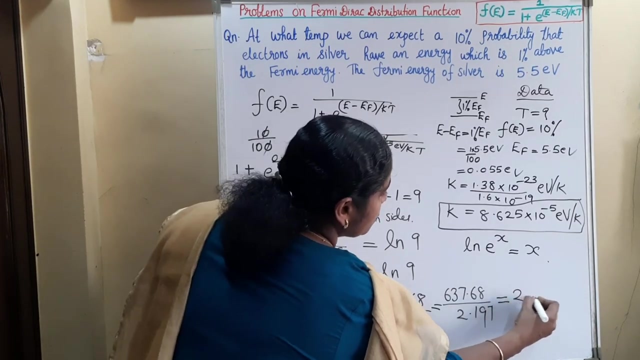 multiply this with the 2.303.. So we will get this as 637.68 divided by t is equal to log 9.. t is equal to 637.68 divided by log 9.. t is 637.68 divided by 2.197 is equal to 290 Kelvin. 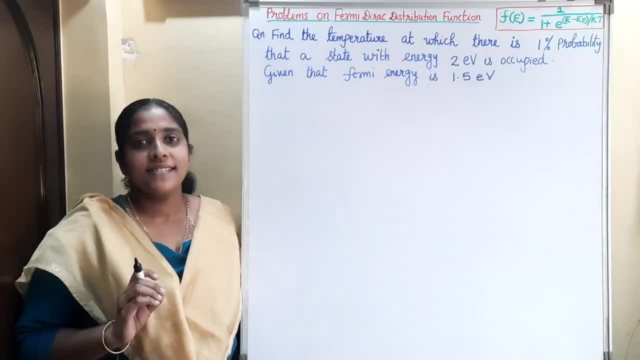 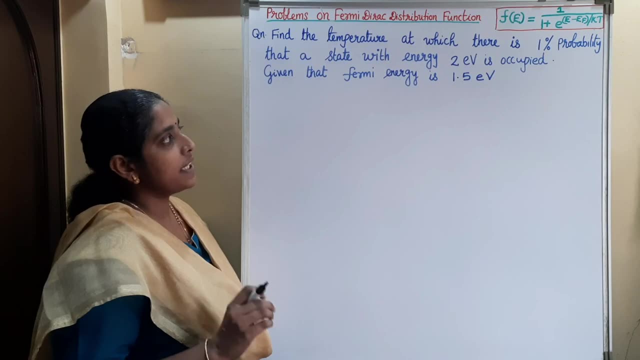 So the temperature for the given question is 290 Kelvin. See this question. See this question. Find the temperature at which there is one percentage probability that a state with the energy 2 electron volt is occupied, given that Fermi energy is 1.5 electron volt. 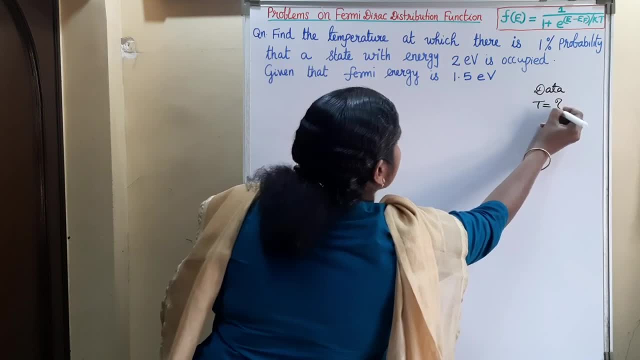 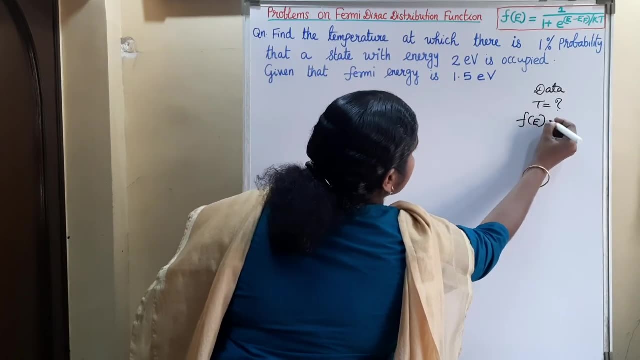 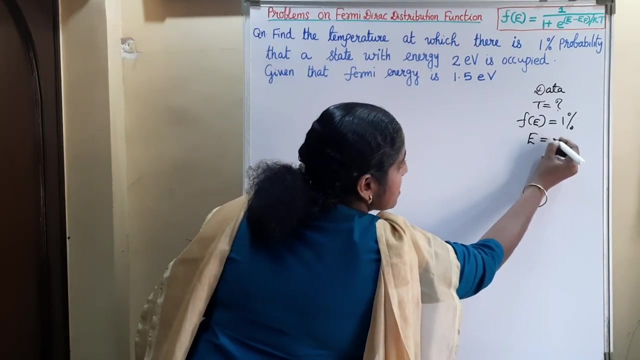 Find the temperature. So we have to find out the temperature at which there is one percentage probability. Probability means the function f of e is equal to one percentage. with energy, 2 electron volt is occupied, So energy level is given as 2 electron volt. 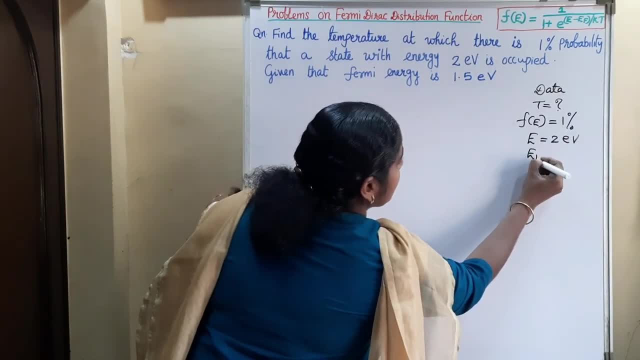 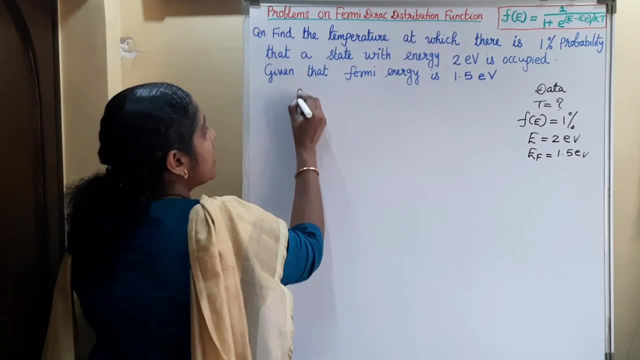 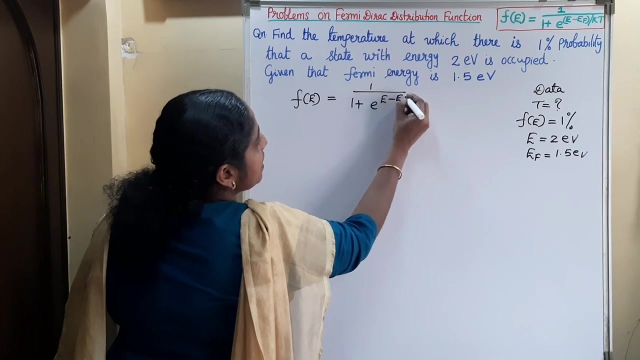 Given that Fermi energy is 1.5 electron volt, So E f is equal to 1.5 electron volt. So we can write the general formula for the Fermi derived distribution function: f of e is equal to 1 by 1 plus E raised to E minus E, f by kT. 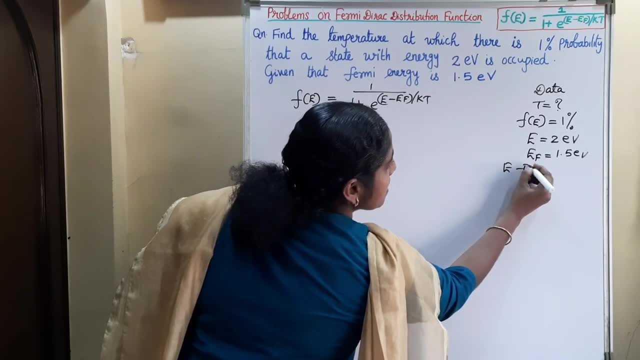 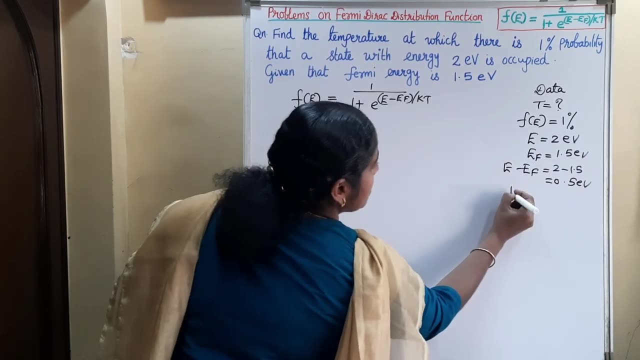 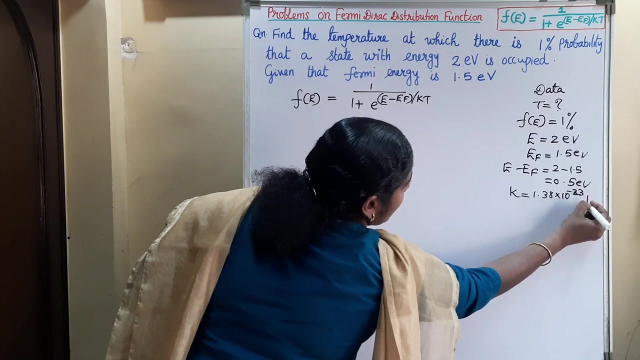 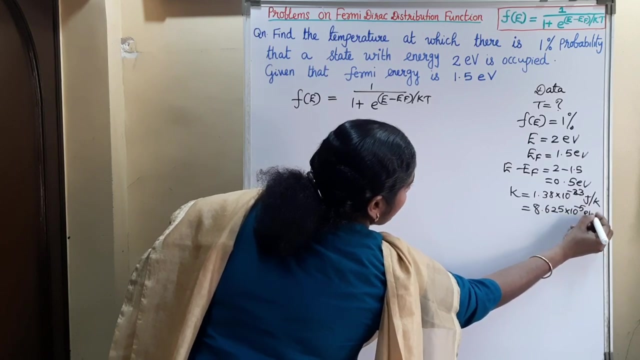 So here E minus E, f is 2 minus 1.5, that is equal to 0.5 electron volt, and k is Boltzmann constant. that is equal to 1.38 into 10 raised to minus 23 joule per kelvin, or in electron volt we can write it as 8.625 into 10 raised to minus 5 electron. 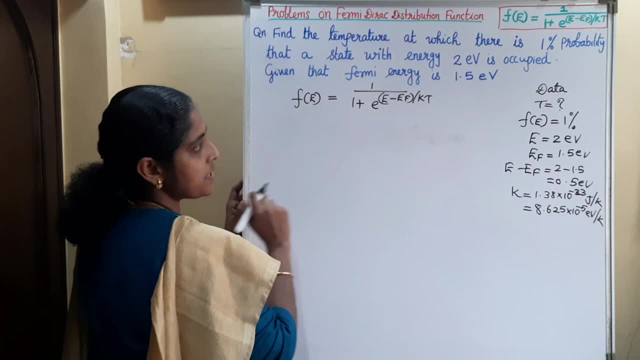 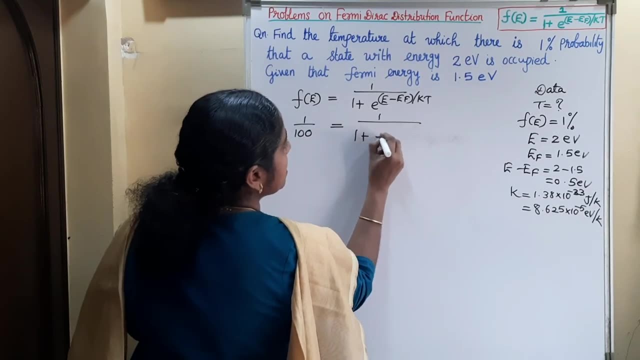 volt per kelvin. Okay, now we can substitute these values here. f of e is equal to 1 percentage, that is, 1 by 100 is equal to 1 by 1 plus e. raised to e minus ef is 0.5 electron volt divided by. 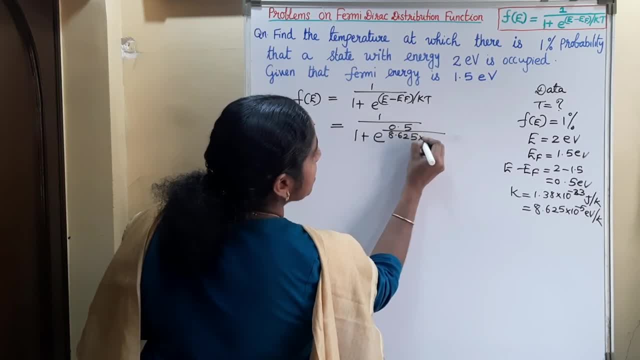 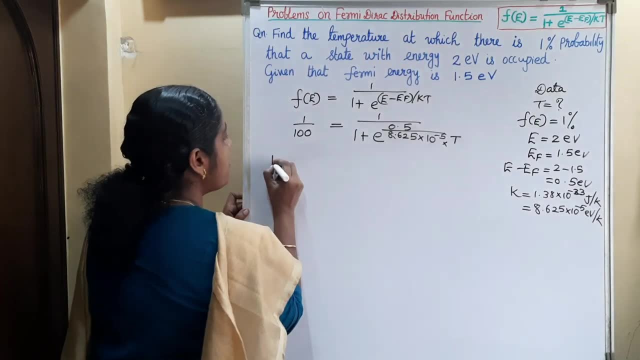 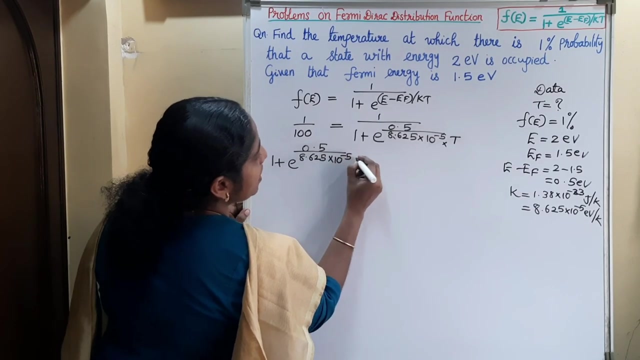 k is 8.625 into 10, raised to minus 5. electron volt per kelvin t. Now on cross multiplying this, 1 plus e, raised to 0.5, divided by 8.625 into 10, raised to minus 5, into temperature equal to 100.. 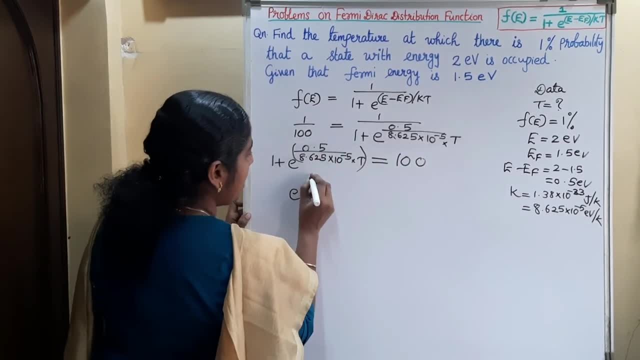 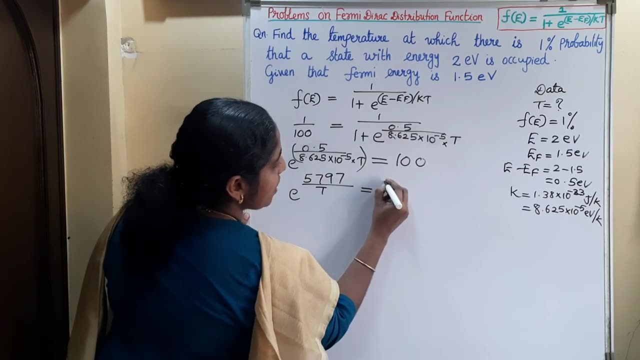 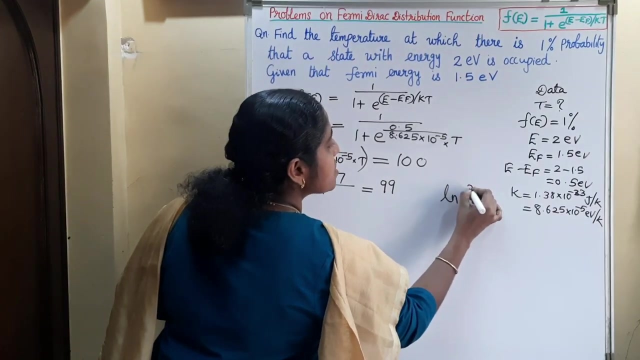 So e raised to- on solving this we will get- 5797 divided by t is equal to this one we can take to that side. so 100 minus 1 is 99. So now we have an exponential here. we know that logarithm of e raised to x is x. so we can remove this exponential by taking the logarithm. 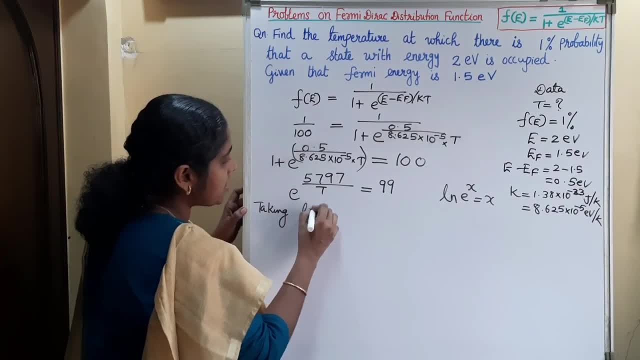 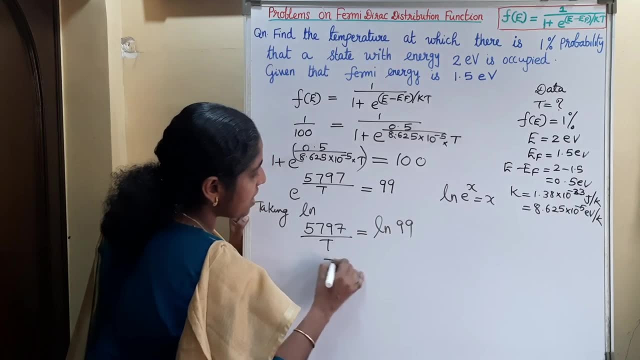 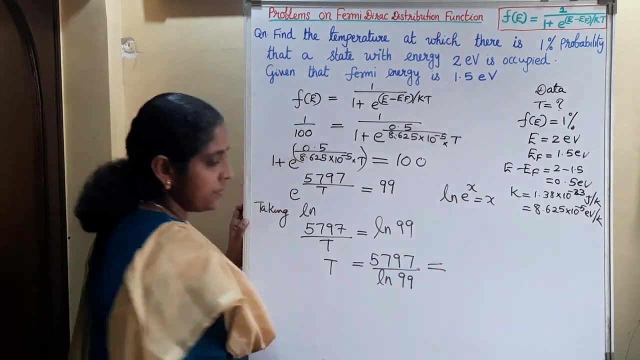 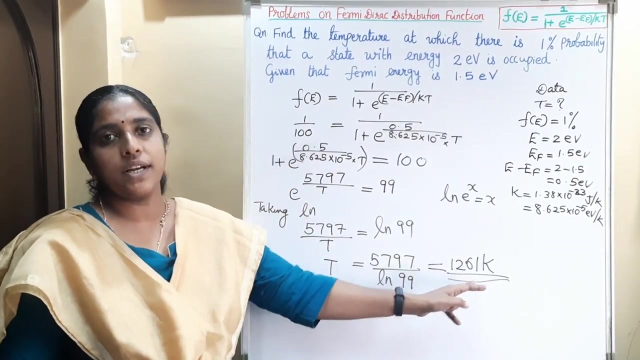 So taking logarithm on both sides, we will get this as 5797 divided by t is equal to logarithm Log 99, or t is equal to 5797 divided by log 99, that is equal to 1261 kelvin. So the temperature for the given question is 1261 kelvin. 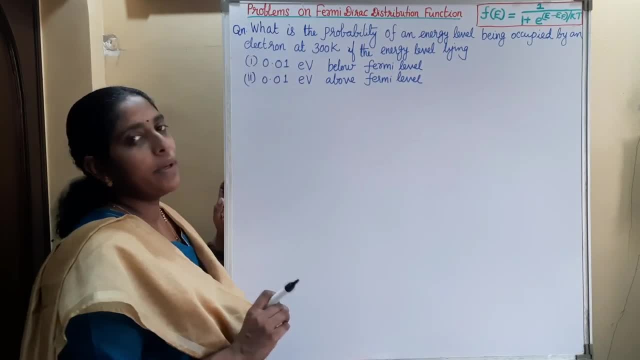 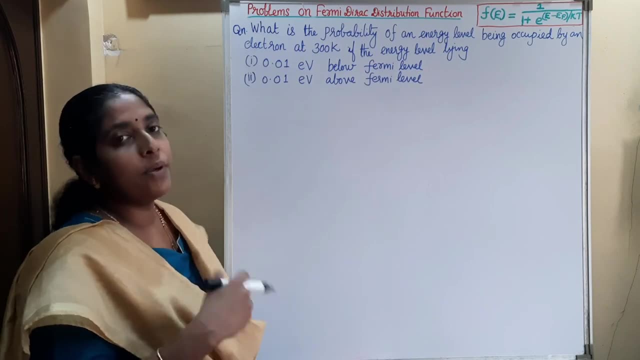 Next question: what is the probability of an energy level being occupied by an electron at 300 kelvin if the energy level lying 0.01 electron volt below the Fermi level? and, in the 2nd case, 0.01 electron volt above the Fermi level? 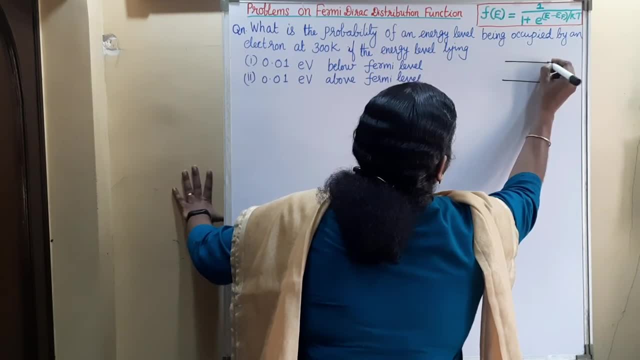 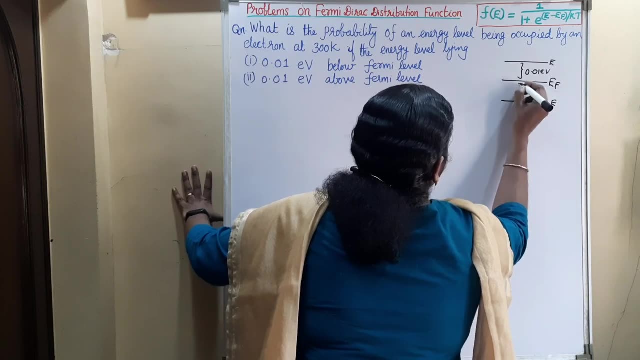 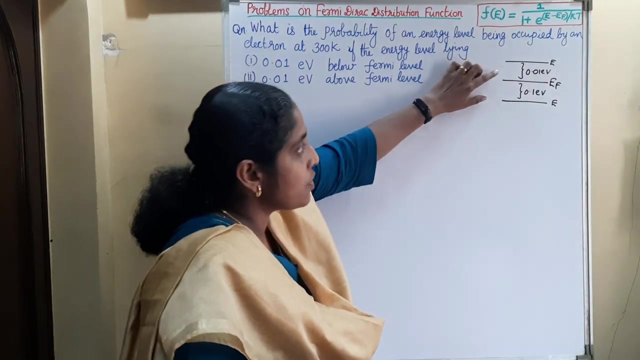 this Fermi level is here. We are considering an energy level that is above Fermi level and we are considering an energy level that is below Fermi level. So we have to find out the probability of occupancy of electron at 0.01 electron volt above the Fermi. 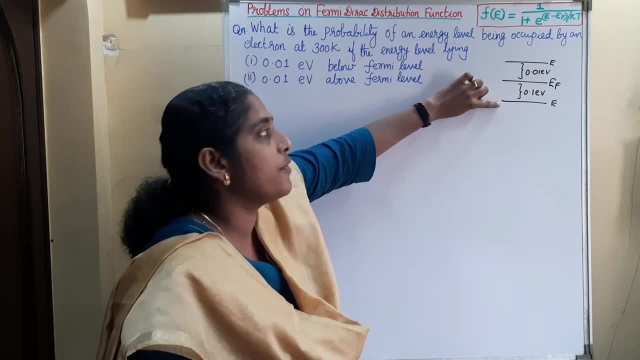 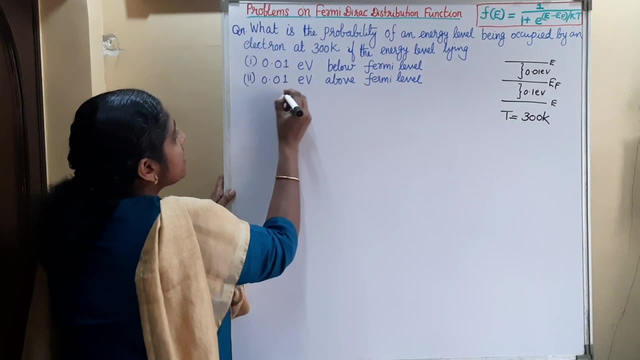 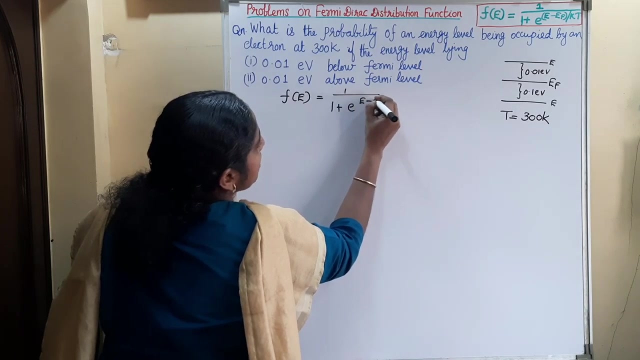 level and at an energy level 0.01 electron volt below the Fermi level, And it is also given that a temperature is equal to 300 Kelvin. So we can write the general formula: F of E is equal to 1 by 1 plus E. raise to E minus EF by kT Above the Fermi level. E minus EF is: 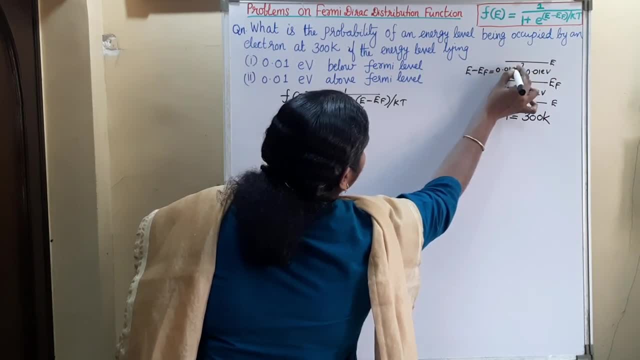 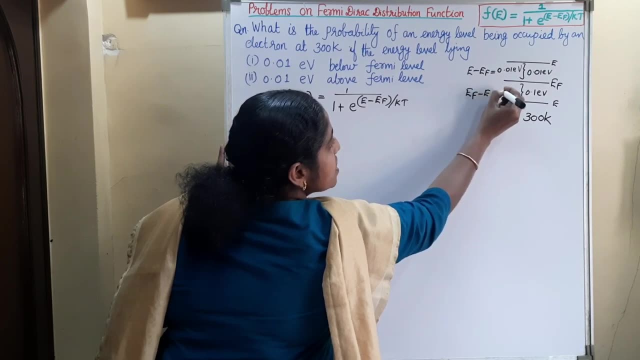 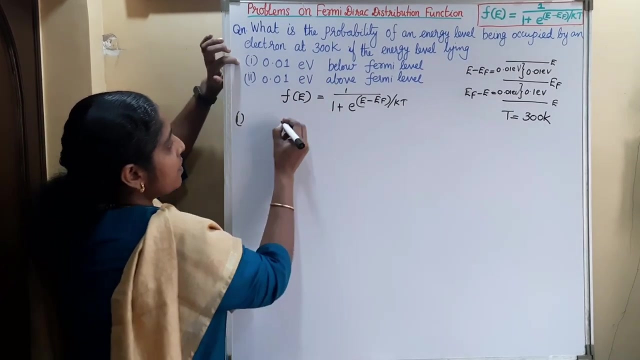 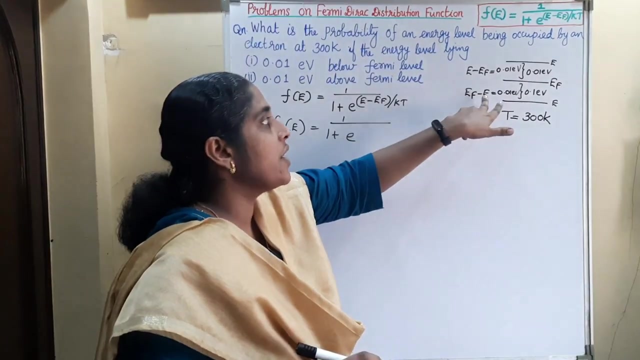 0.01 electron volt. So while we consider the energy level below Fermi level, that is EF minus E equal to 0.01 electron volt. So we can consider the first case 0.01 electron volt below the Fermi level. So F of E is equal to 1 by 1 plus E raise to below Fermi level: EF minus E. 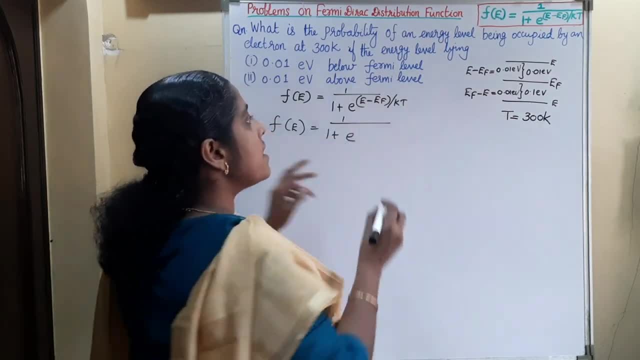 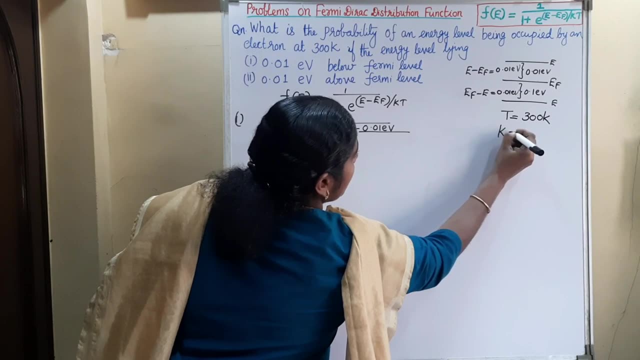 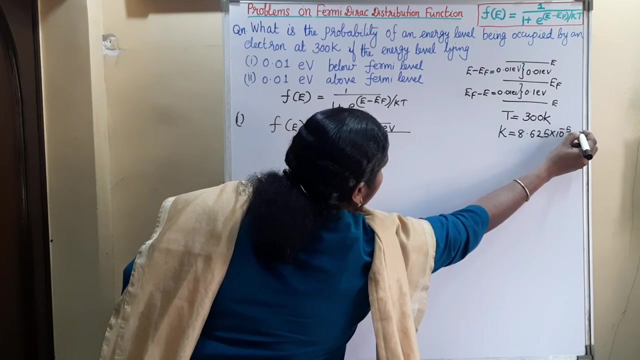 is 0.01 electron volt. So E minus EF is minus 0.01 electron volt divided by kT. What is k? Boltzmann constant, 8.625.. Into 10, raised to minus 5 electron volt per Kelvin, and kT is equal to multiply this with. 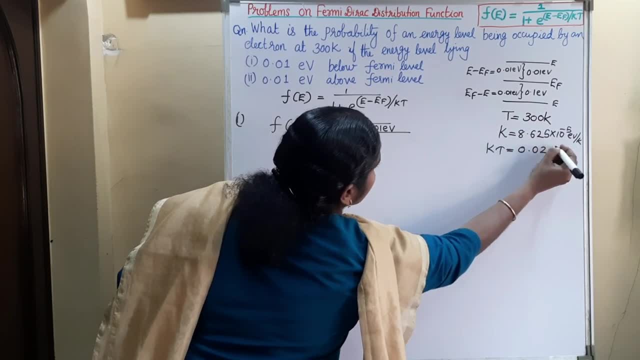 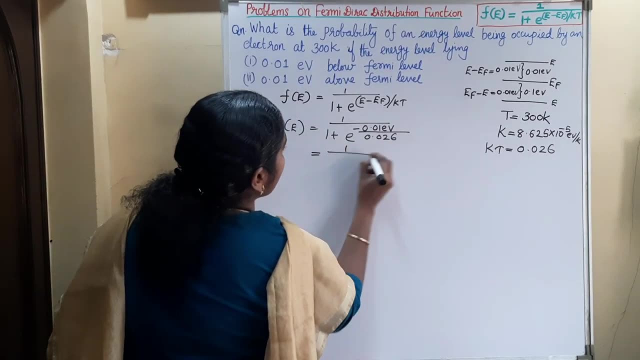 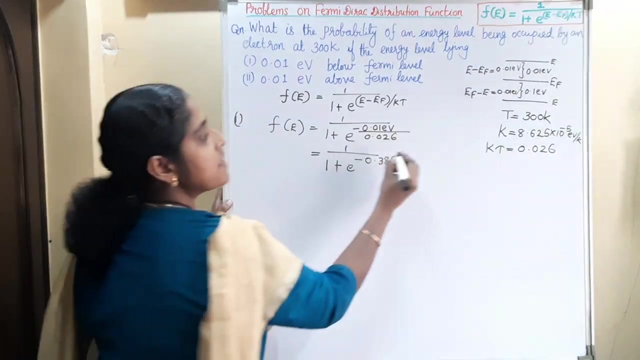 300 Kelvin, we will get 0.026.. So on calculating this, we will get 1 by 1 plus it is E raised to minus 0.3865.. On calculating this, we will get 0.595.. So this is the probability of occupancy. 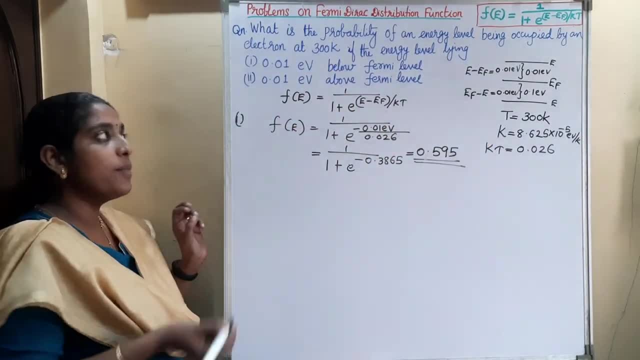 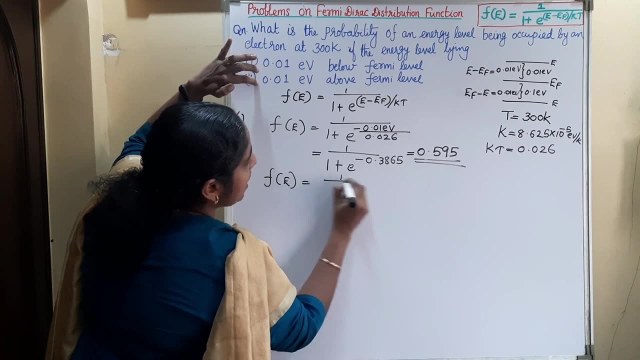 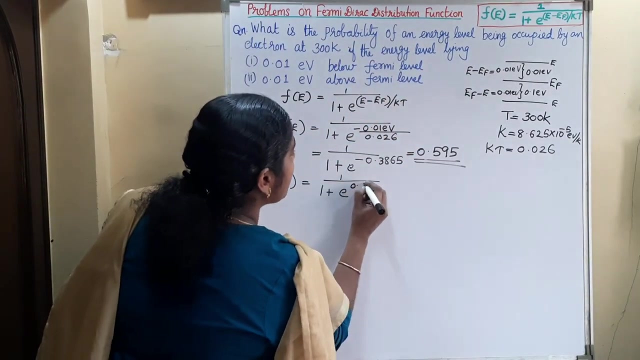 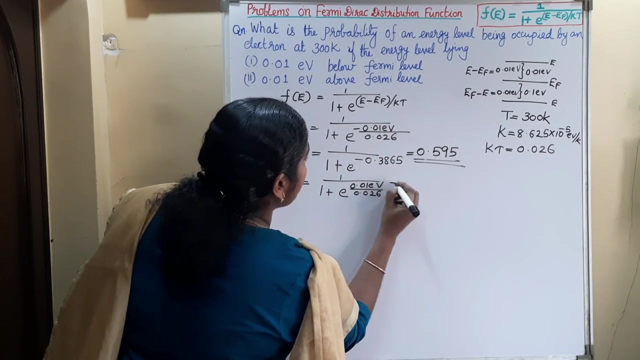 At an energy level which is 0.01 electron volt below Fermi level. Second case is above Fermi level, So that time we will get: F of E is equal to 1 by 1 plus E raise to E minus EF, that is positive 0.01 electron volt divided by kT, that is kT is 0.026.. So we will get. 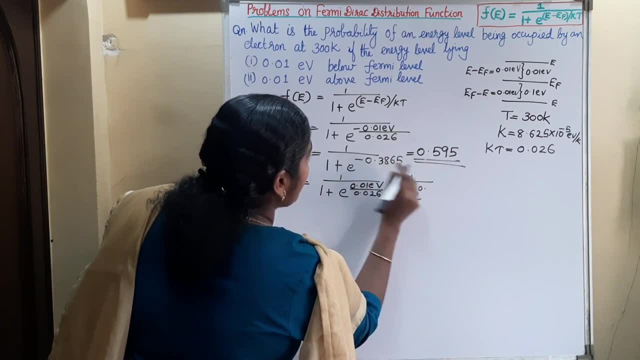 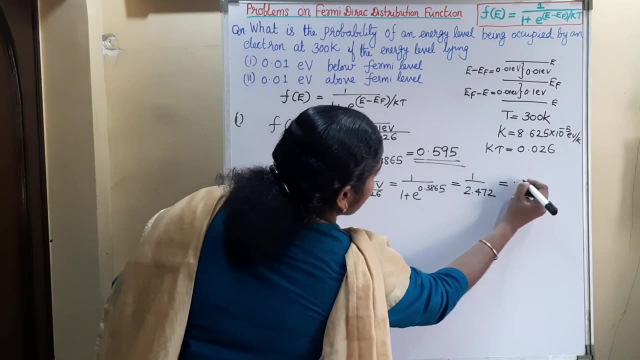 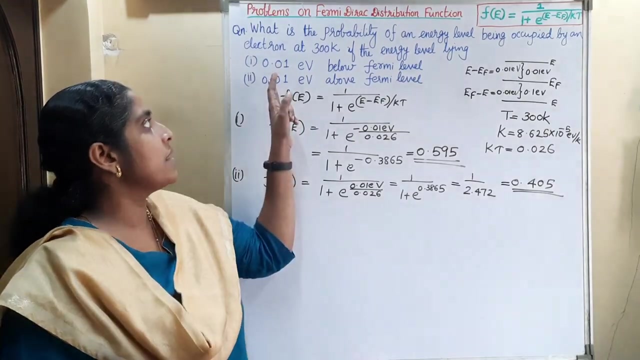 1 by 1 plus E, raise to 0.3865.. So on calculating this we will get 1 by 2.472, that is equal to 0.405.. So this is the probability of occupancy at an energy level 0.01 electron volt above the fermi level. See this Here. 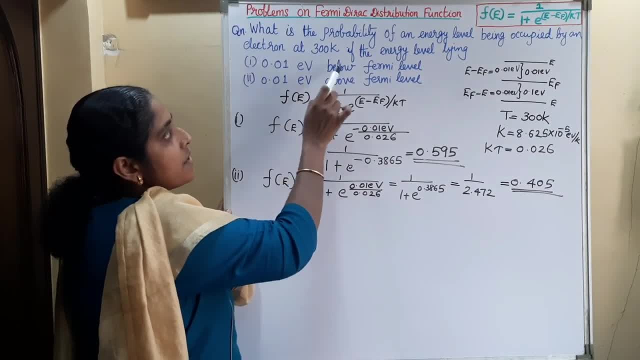 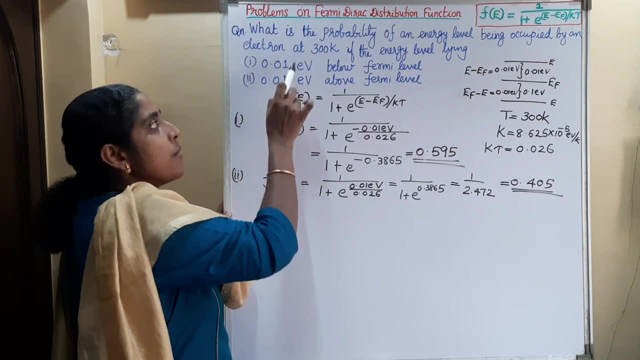 the probability occupancy of energy level which is below the Fermi level is 0.595 and above the Fermi level is 0.405.. Both the energy levels are point 0.255, and so which is the energy number that K is indicating? So we will get 1 by 2.045 and K is the energy level upon this path. Also, Eām is the P gym. What is P omqс? This varies from moment to moment. Here, k matters are equal to e to the. 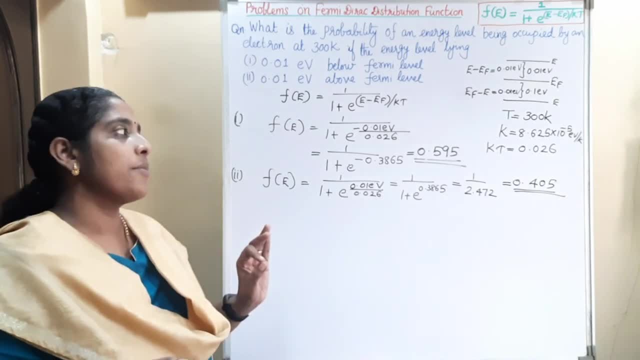 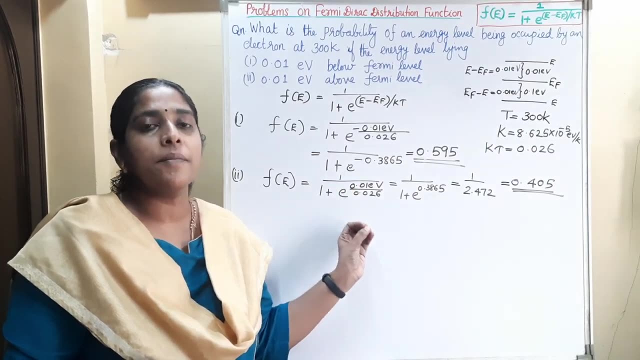 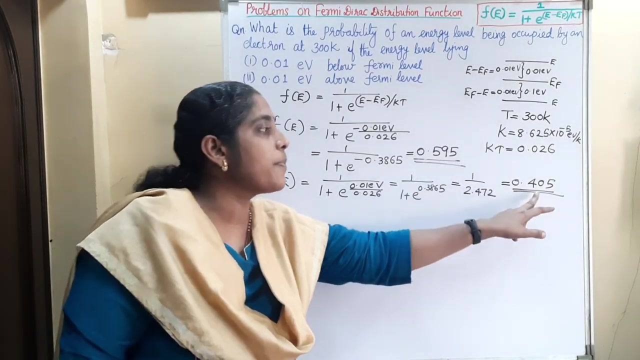 electron volt from the Fermi level. So it is a very important point. The probability occupancy of two energy levels which are equally spaced from the Fermi level, above and below each, will be add up to 1.. See this: 0.595 plus 0.405 is equal to 1.. So probability occupancies of 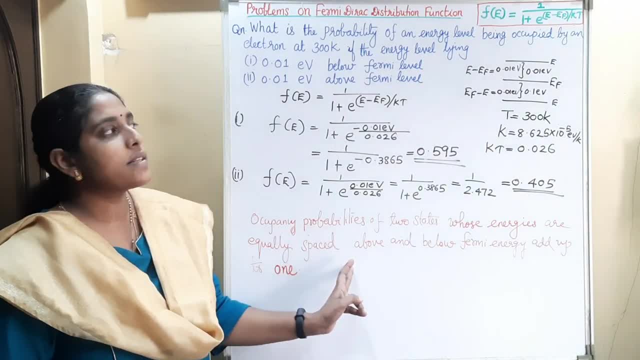 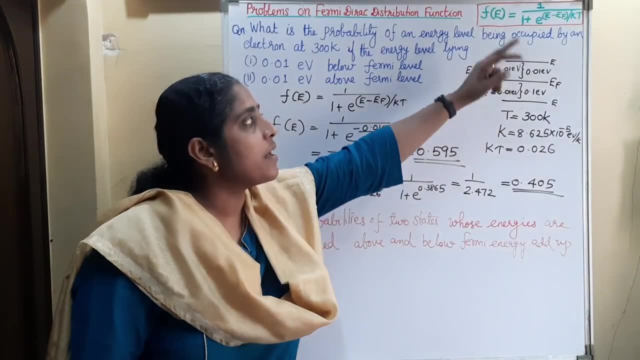 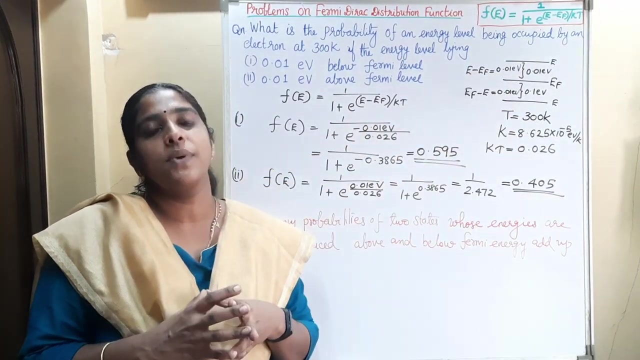 two states whose energies are equally spaced above and below Fermi energy add up to 1.. So if we are taking any energy level above the Fermi level and if the equal spacing energy level we are considering below the Fermi level, both of the probability occupancy will be add to. 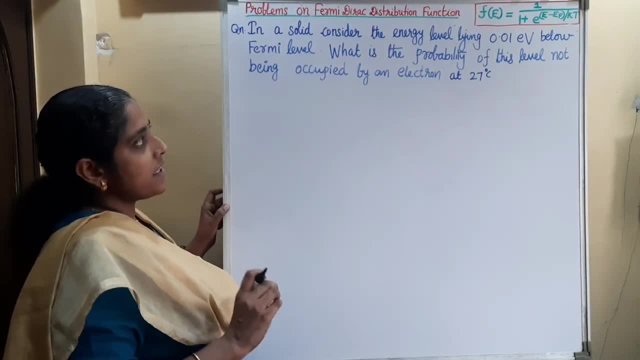 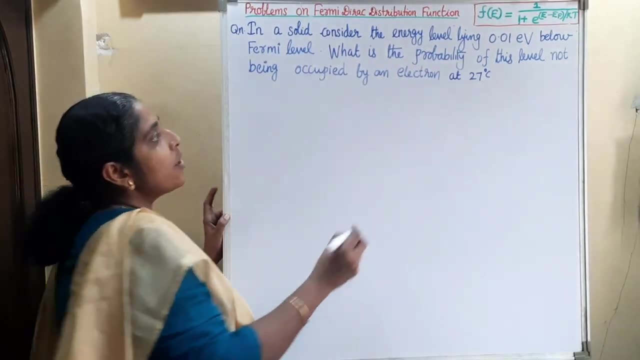 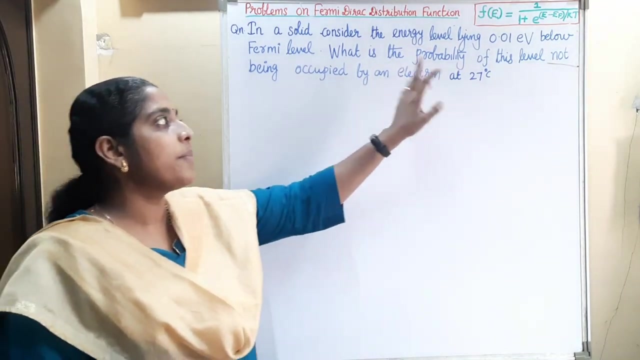 1.. Next question: In a solid, consider the energy level lying 0.01 electron volt below Fermi level. What is the probability of this level not being occupied by an electron at 27 degree Celsius? So we have to find out the probability. 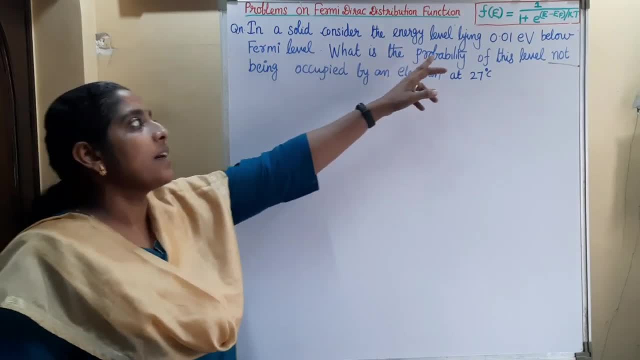 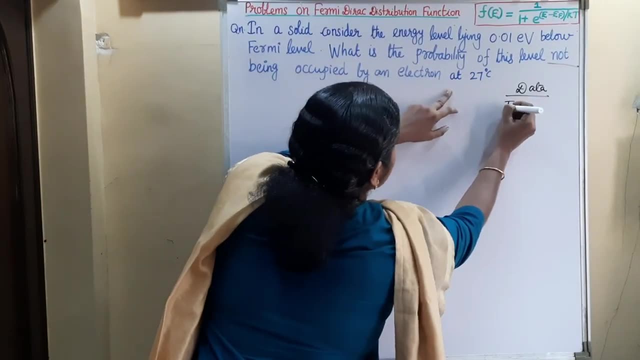 of the energy occupancy of two states which are equally spaced above and below the Fermi level, The probability of not occupying the electron for this energy level 0.01 electron volt below the Fermi level. So it is given that the temperature T is equal to 27 degree Celsius. 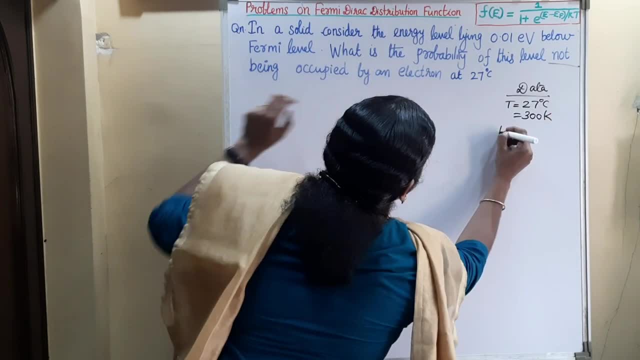 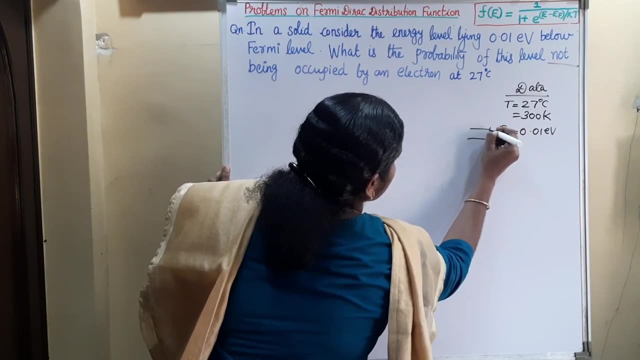 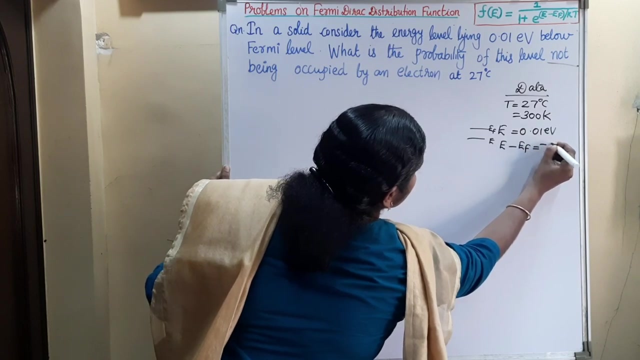 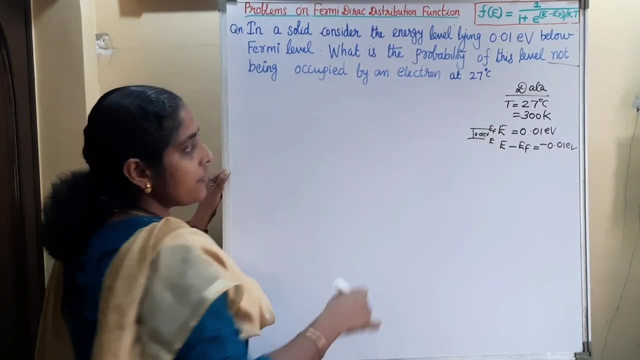 that is 300 Kelvin and the energy level E is equal to 0.01 electron volt below the Fermi level. So that means E minus EF is equal to minus 0.01 electron volt below the Fermi level. So this is 0.01 electron volt. So this is 0.01 electron volt. energy level is below the Fermi level. 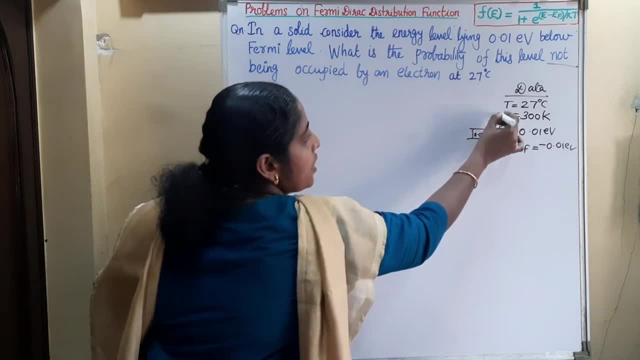 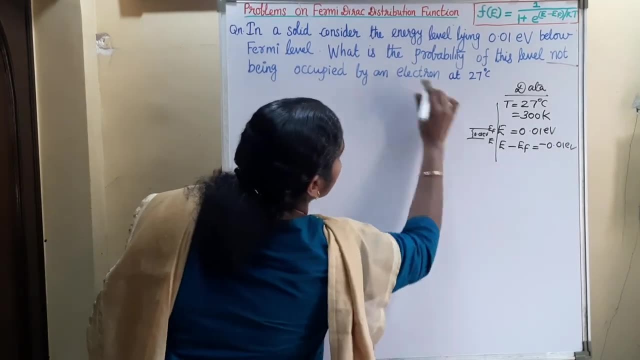 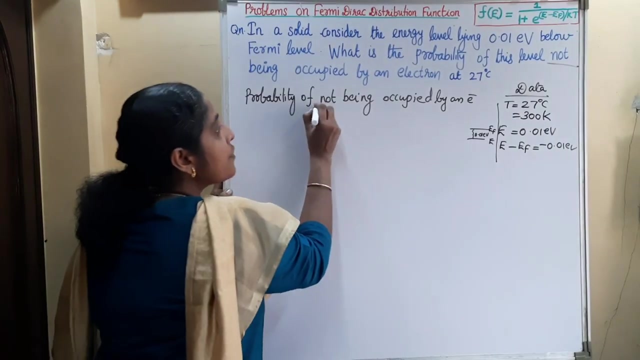 that is, EF minus E is 0.01 electron volt, or E minus EF is minus 0.01 electron volt. So we want to find out the probability of this level not being occupied. So here we have to find out the probability of not being occupied by an electron, The probability of being occupied by. 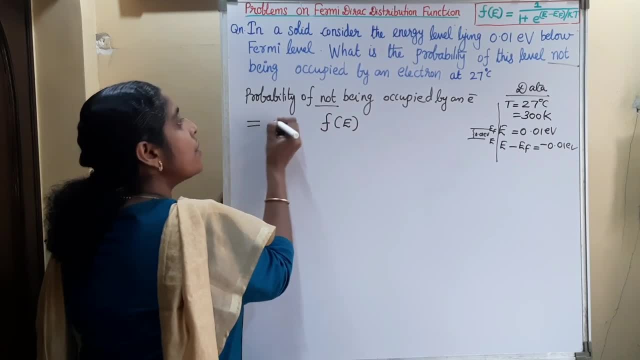 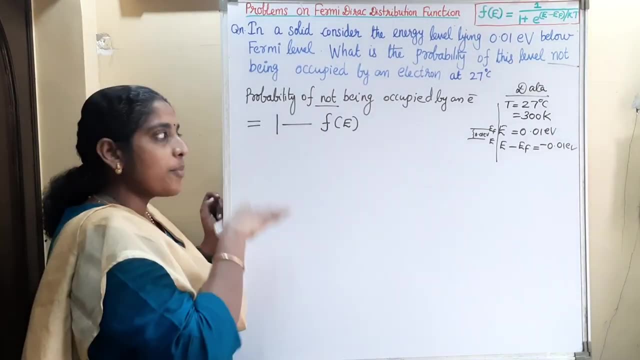 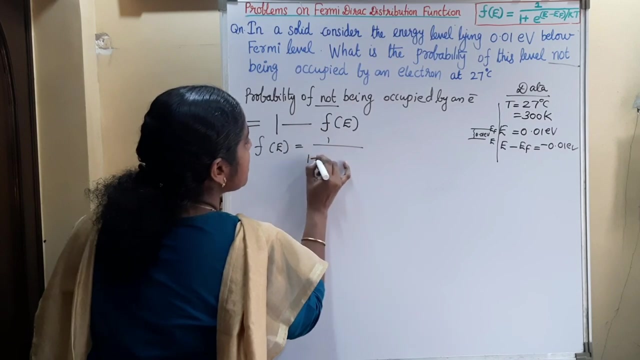 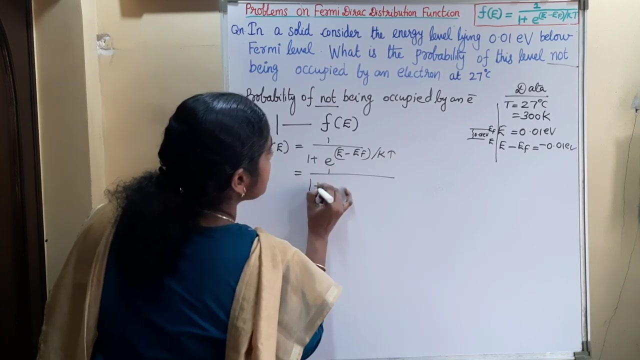 an electron is FOV, So the probability of not being occupied by an electron will be 1 minus FOV. So first we can find out the FOV, then the probability of not occupying is 1 minus FOV. So FOV is equal to 1 by 1 plus E. raised to E minus EF by KT, that is equal to 1 by 1 plus E. 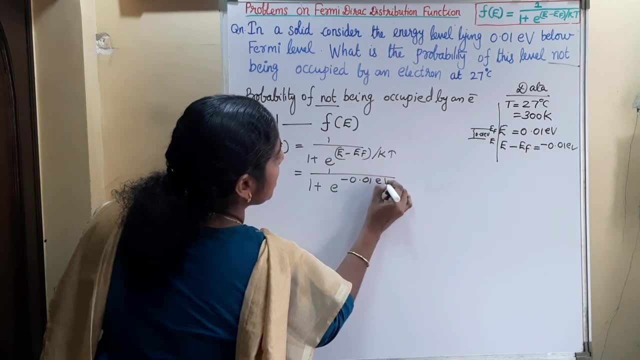 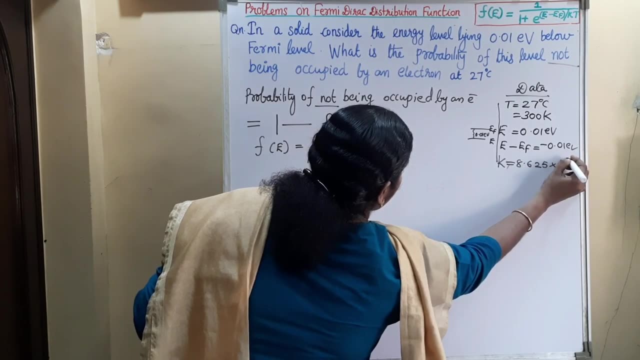 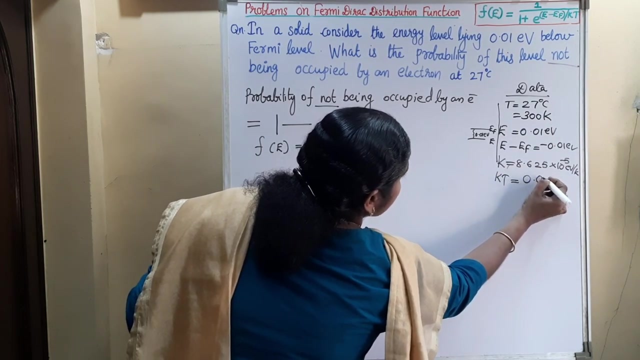 raised to E minus EF is minus 0.01 electron volt. divided So E by K is 8.625 into 10. raised to minus 5 electron volt per Kelvin and KT is room temperature 27 300 Kelvin. So I am doing we will get 0.026.. So we can write here 0.026 electron volt. 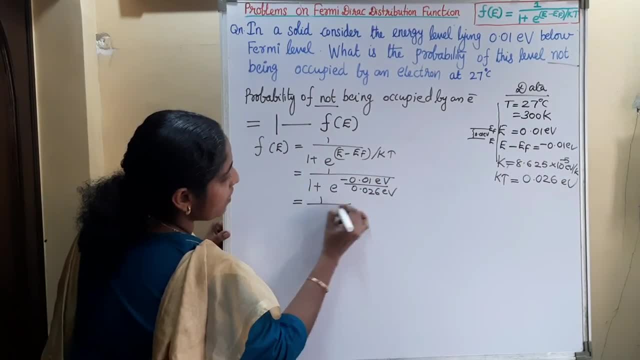 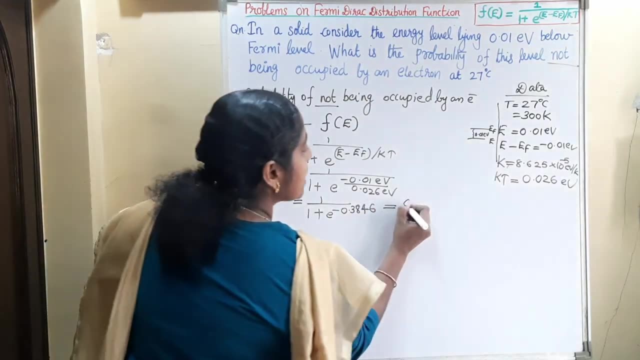 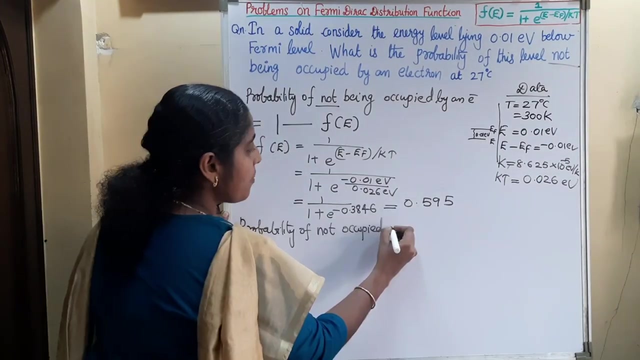 So that is 1 by 1 plus E, raised to minus 0.3846.. So on calculating this we will get 0.026.. So the probability of not being occupied is 1 minus FOV. So probability of not occupied is: 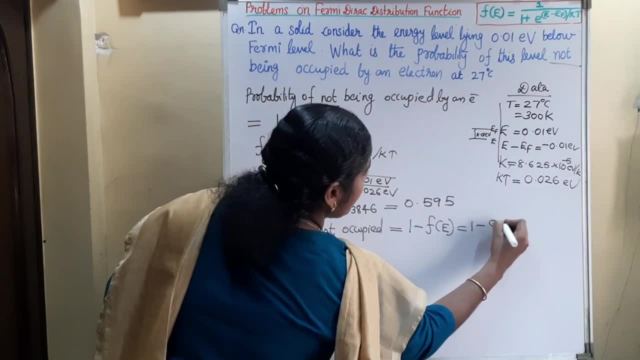 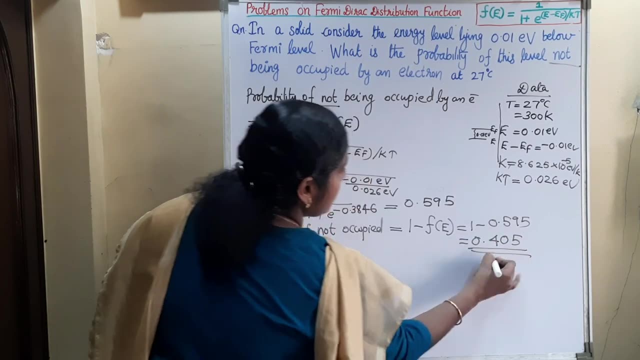 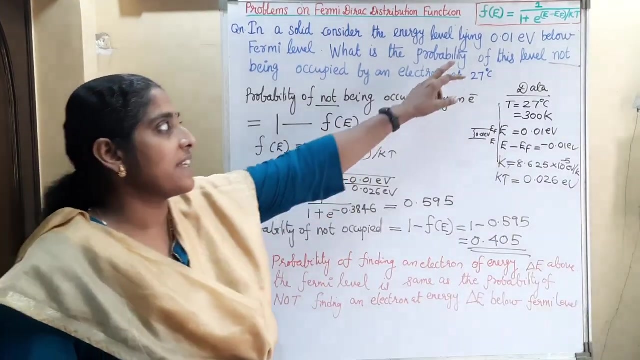 1 minus FOV, that is 1 minus 0.595, that is 0.405.. So the answer is 0.405.. In the previous question we have discussed the probability of occupancy of an energy level which is 0.01 electron volt lying. 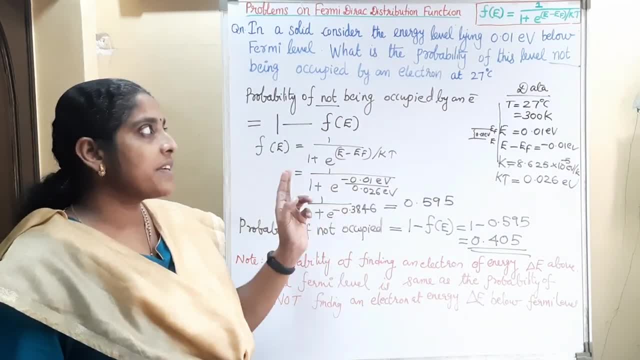 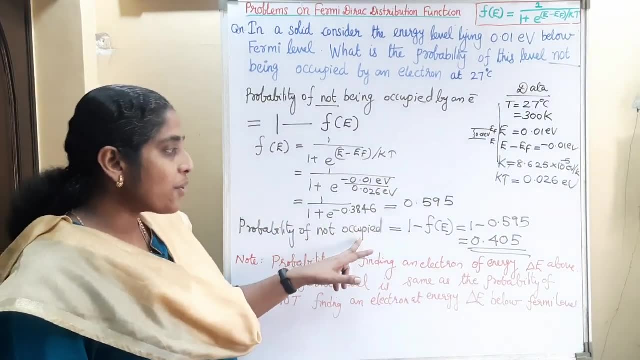 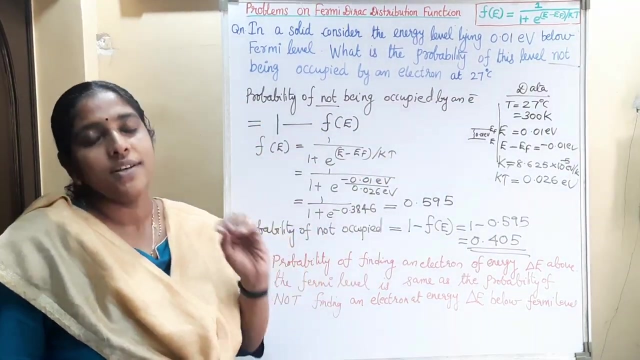 Above the Fermi level and below the Fermi level. Then we considered: above the Fermi level, we got the answer 0.405.. Now the probability of not occupying in an energy level 0.01 electron volt below the Fermi level is 0.405.. So it is an important point, that is, probability of finding. 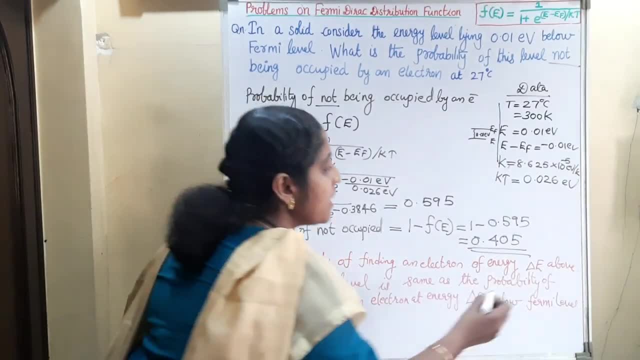 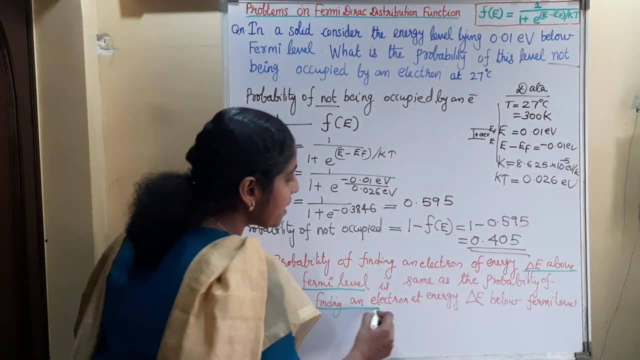 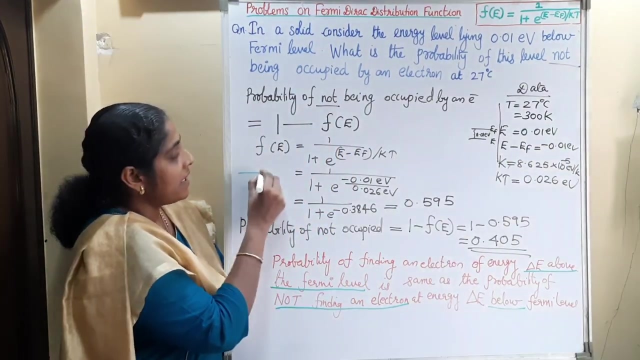 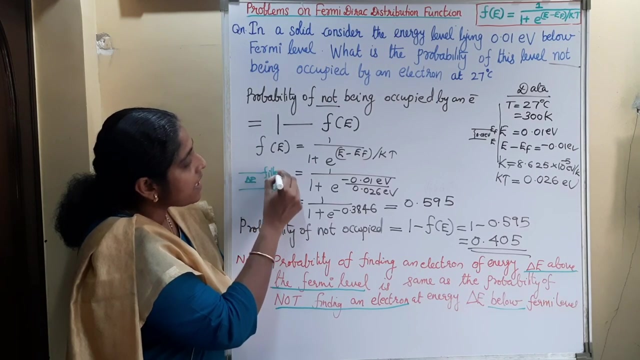 an electron of energy delta E above the Fermi level is same as the probability Of not finding an electron at the energy level delta E below the Fermi level. or we can say that an energy level delta E above the Fermi level which is filled is same as an energy level delta E. 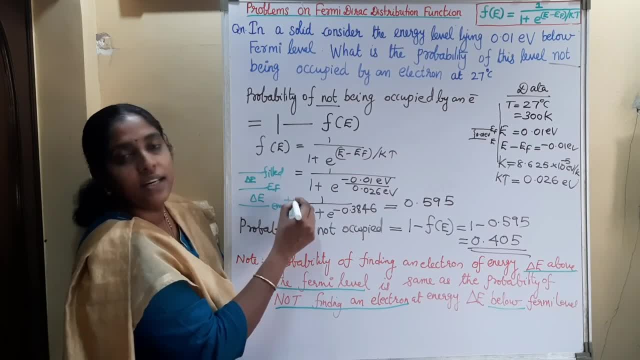 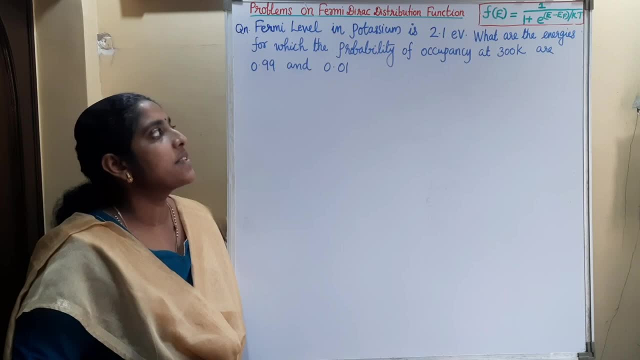 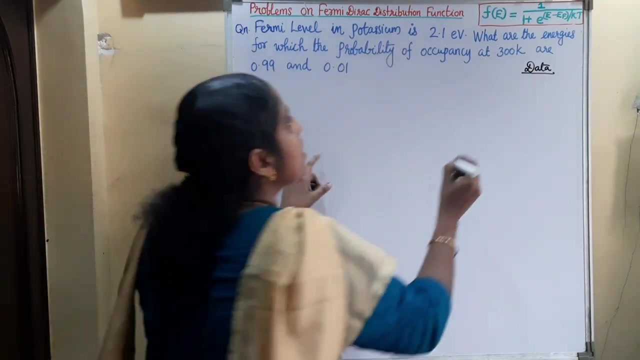 below the Fermi level, which is empty. One last question. Fermi level in potassium is 2.1 electron volt. What are the energies formed? What are the energies formed? What are the energies formed For which the probability of occupancy at 300 Kelvin are 0.99 and 0.01.. It is given Fermi level is: 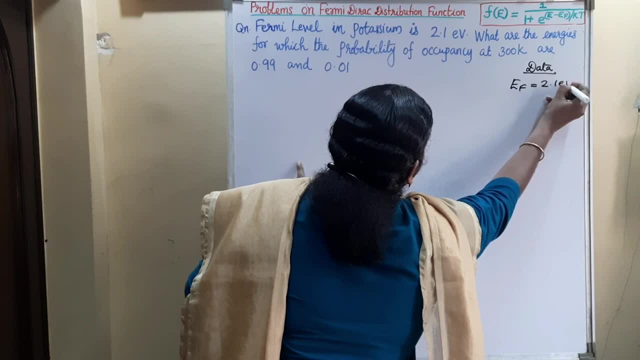 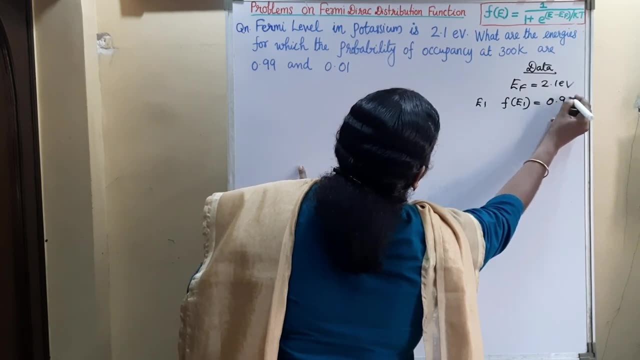 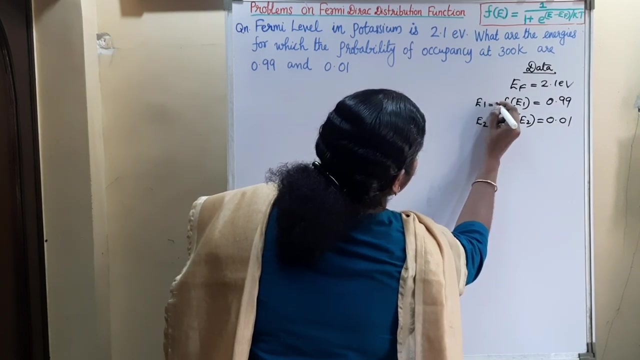 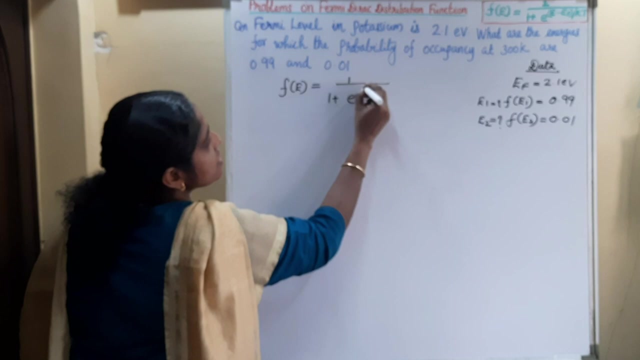 2.1 electron volt. What are the energies for which the probability of occupancy at 300 Kelvin are 0.99 and 0.01.. So we have to find out the energy in which the given probability, Therefore form E, is equal to 1. by 1 plus e raise to e minus ef. by kT Temperature is given as 300 Kelvin. 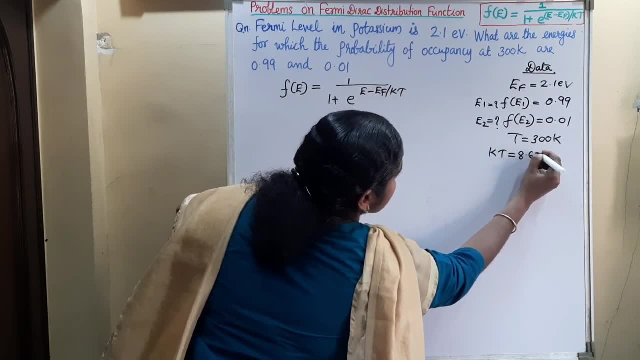 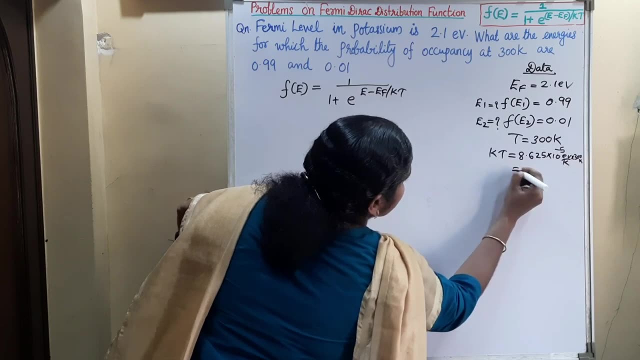 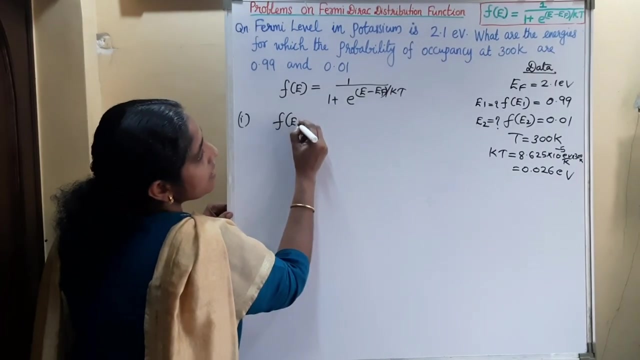 So kT is equal to 8.625. into 10, raise to minus 5 electron volt per Kelvin into 300 Kelvin, That is equal to 0.026 electron volt. So first case F of E 1 is equal to 1. 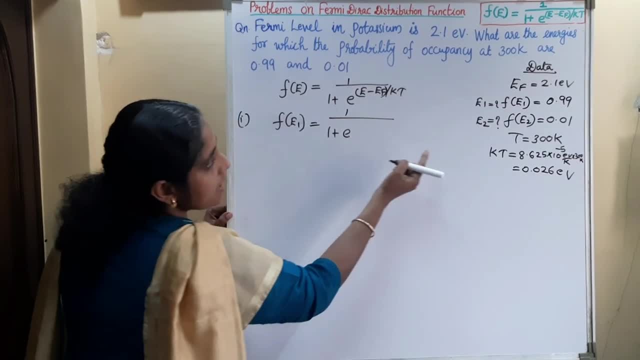 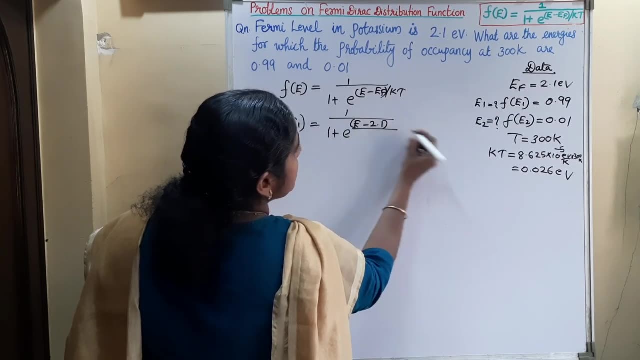 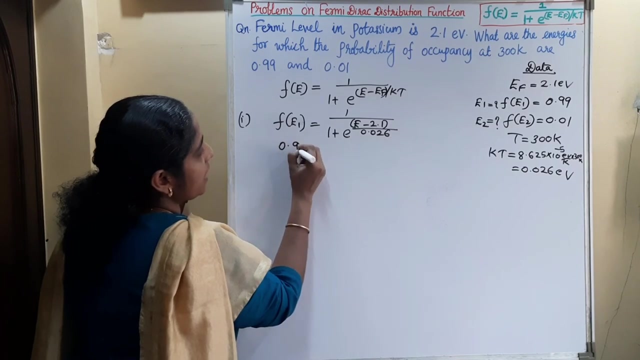 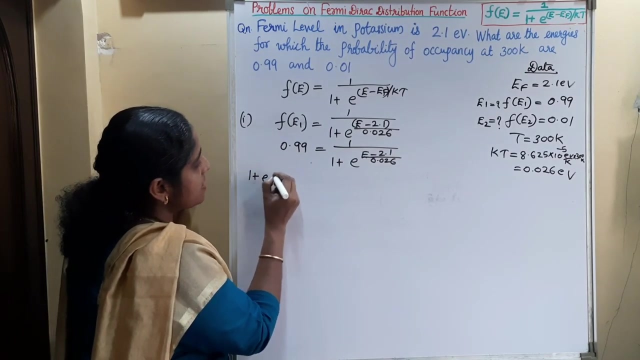 by 1 plus e, raised to e minus ef, so e minus 2.1 electron volt. divided by kt, kt is 0.026 electron volt, so f of e1 is 0.99. is equal to 1 by 1 plus e so on cross multiplying here we will get 1 plus. 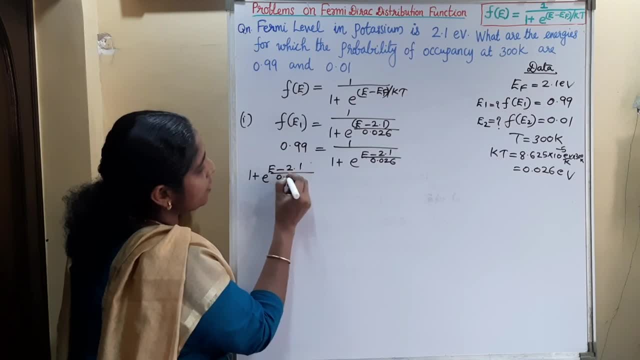 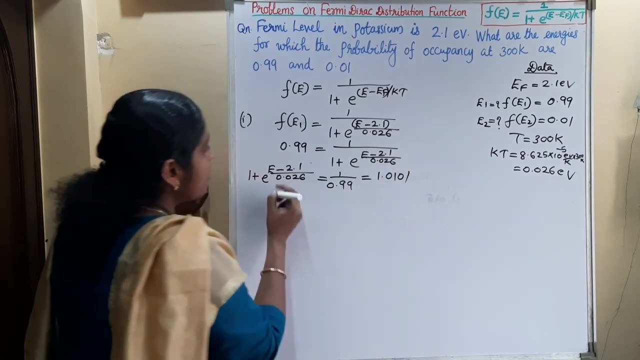 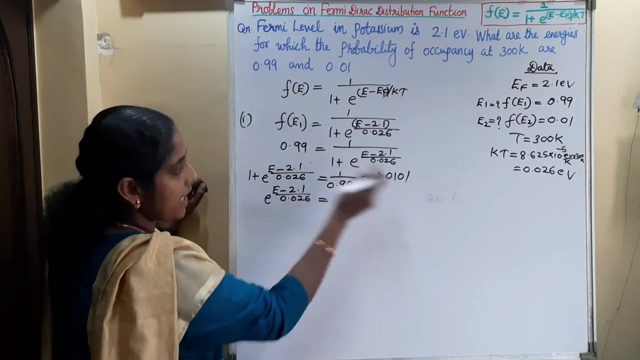 e raised to e minus 2.1, divided by 0.026 equal to 1. by 0.99, this equal to 1.0101. or we can write this as: e raised to e minus 2.1 by 0.026. when we can take to that side, so minus 1 that is 0.0101. 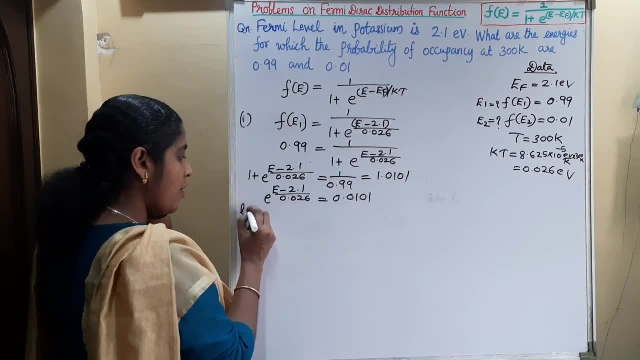 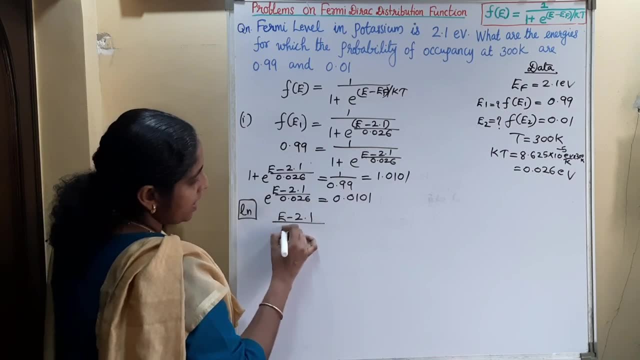 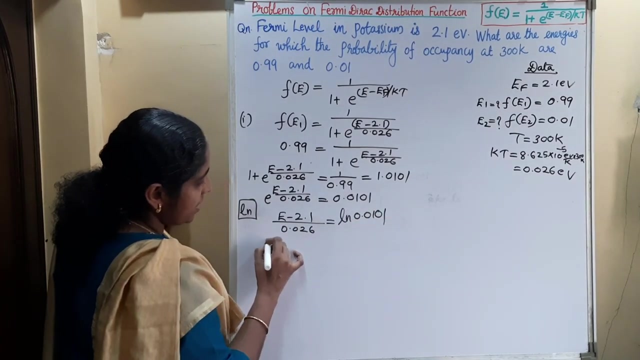 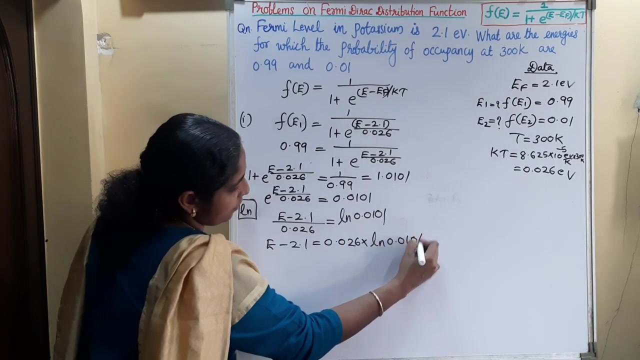 or on taking logarithm on both side, so that this exponential we can remove, so we can write it as e minus 2.1 by 0.026 equal to log 0.0101, or e minus 2.1 is equal to 0.026 into log 0.0101. so on calculating, 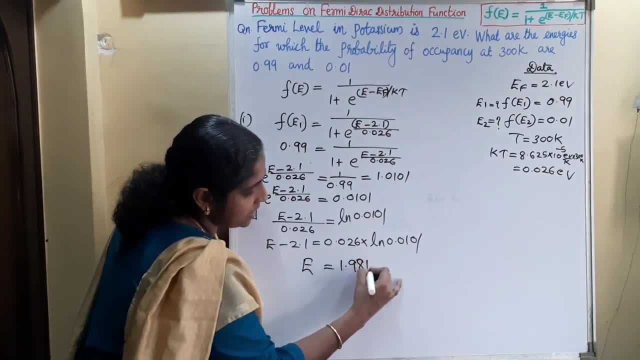 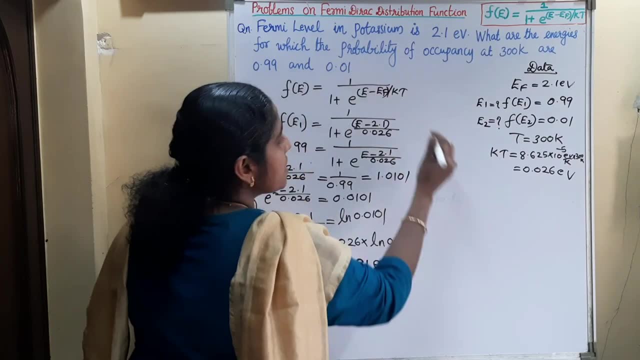 this we will get. e is equal to 1.981 electron volt. the second part: we have to find out the energy level for which the probability is 0.01. so here in the general expression is 0.01. so here in the general expression is 0.01. so here in the general expression. 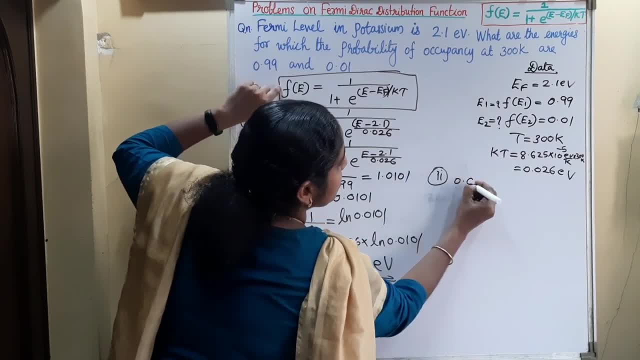 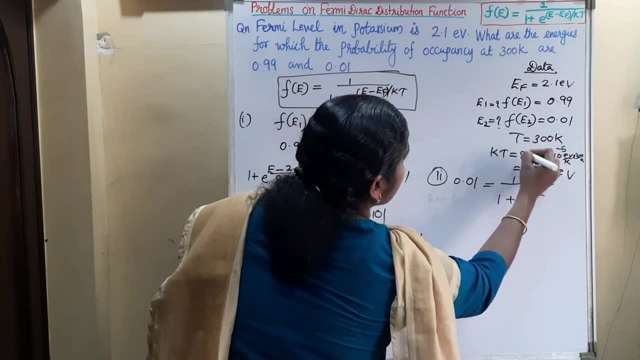 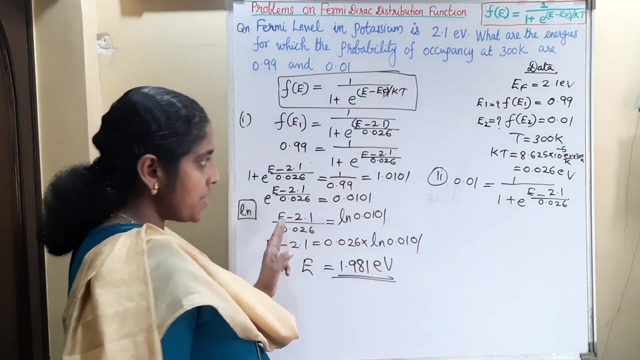 F of E is equal to 0.01, that is equal to 1 by 1 plus E raise to E minus EF is 2.1 electron volt divided by KTE 0.026.. So similar to this, we can cross, multiply and solve. So 1 plus E raise to. 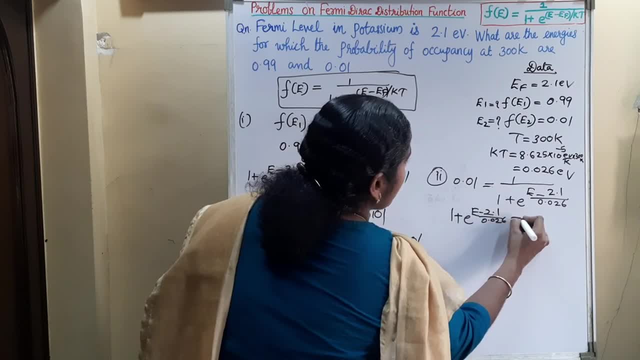 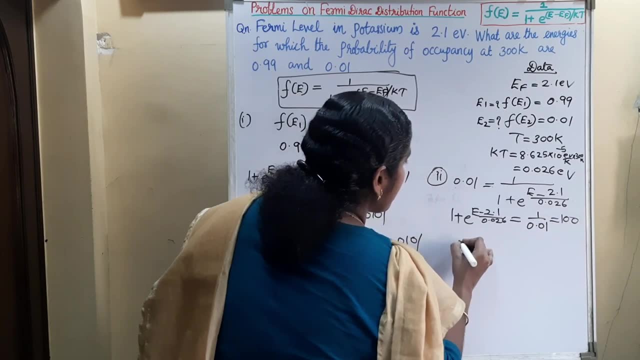 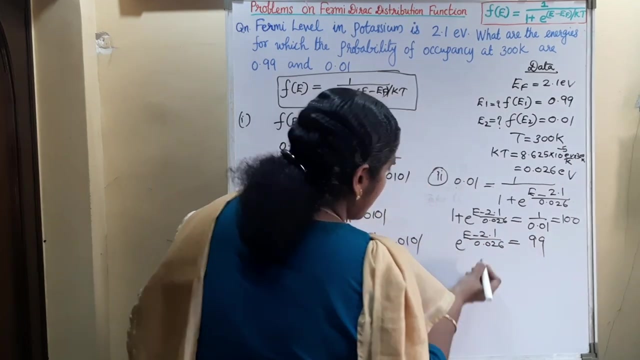 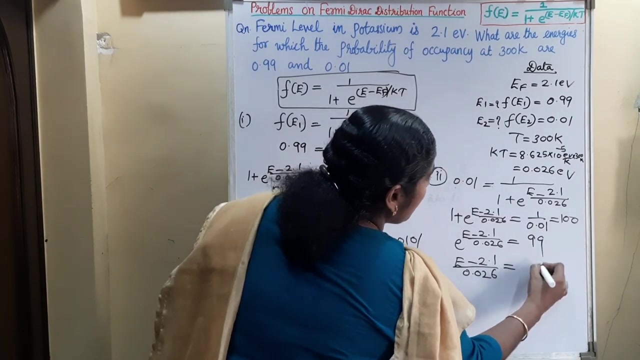 E minus 2.1 by 0.026 equal to 1. divided by 0.01, that is equal to 100.. So E raise to E minus 2.1 by 0.026 is equal to 99, or taking the logarithm, we will get E minus 2.1 by 0.026 equal to log 99.. 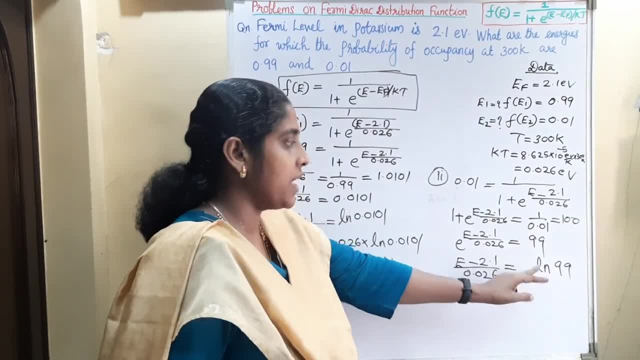 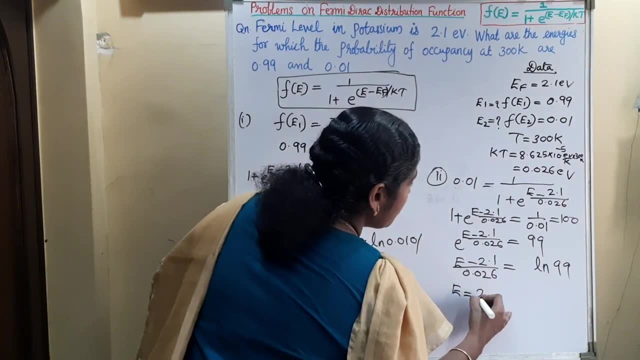 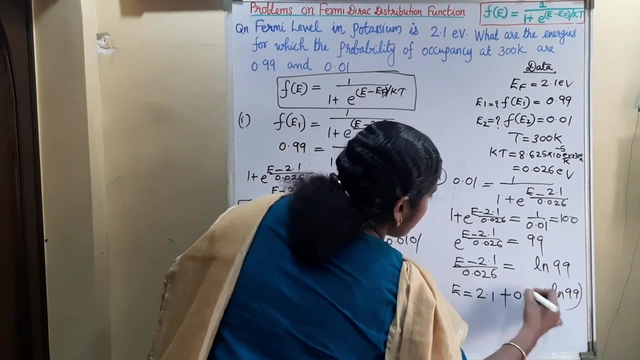 Remember we have to take the natural logarithm. If you are taking base test Logarithm, multiply that with the 2.303.. So E is equal to 2.1 plus 0.026 log 99. So on. 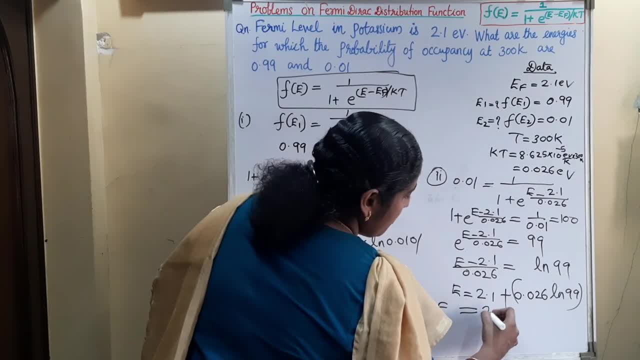 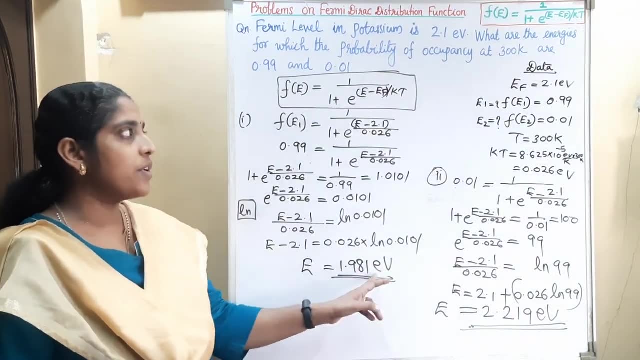 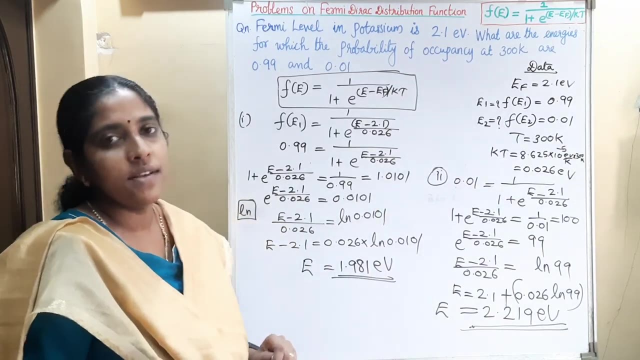 calculating this, we will get this energy as 2.219 electron volt. So at a 1.981 electron volt, the probability of occupancy is 0.99 and at a 2.219 electron volt, the probability of occupancy is 0.01 electron volt. So you try more questions, all the best.